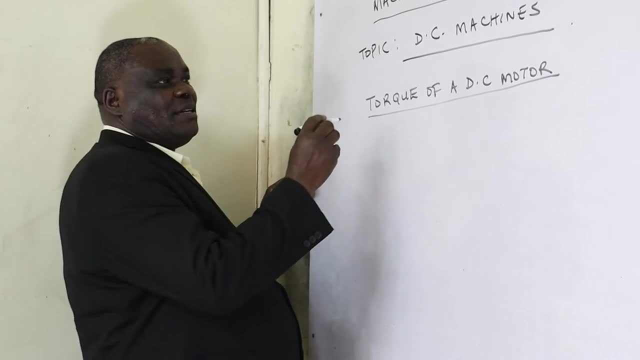 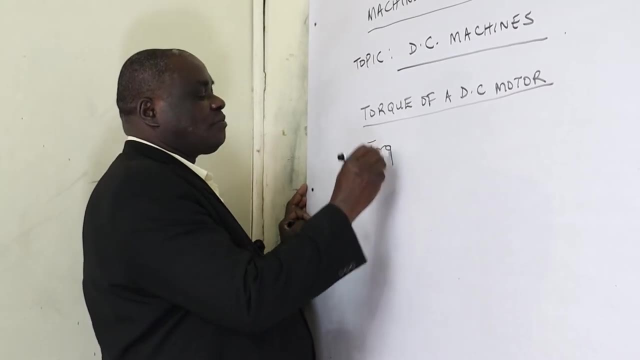 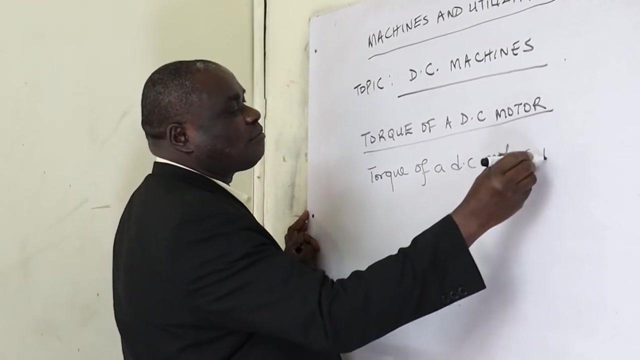 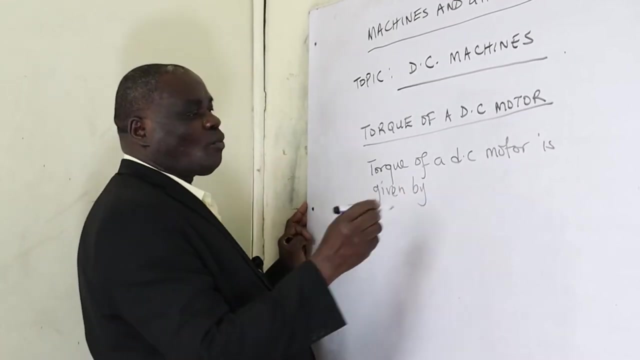 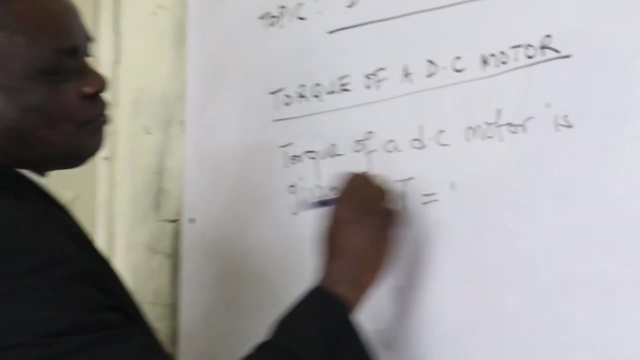 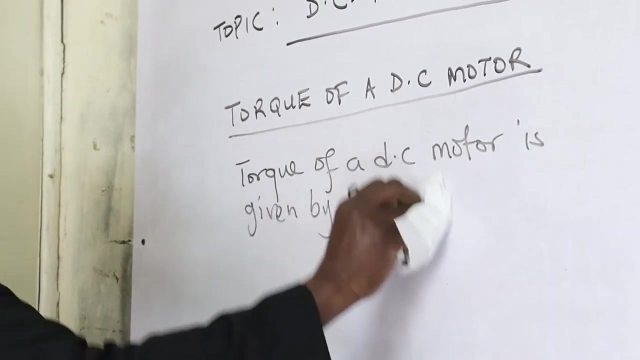 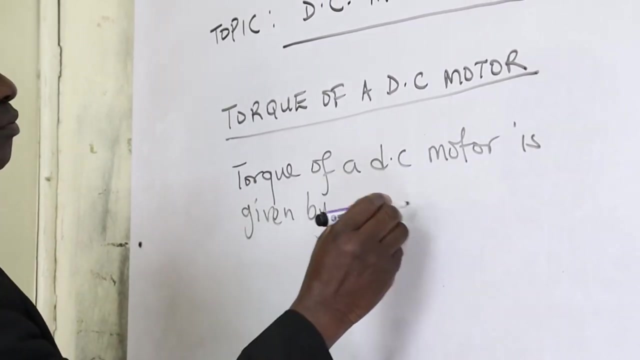 So talk over. DC motor is given by DC motor. This is where, for somebody who is doing diploma in electrical engineering, power option should start from in module 3.. So talk over. DC motor is given by DC motor. This is where, for somebody who is doing diploma in electrical engineering, power option should start from in module 3.. 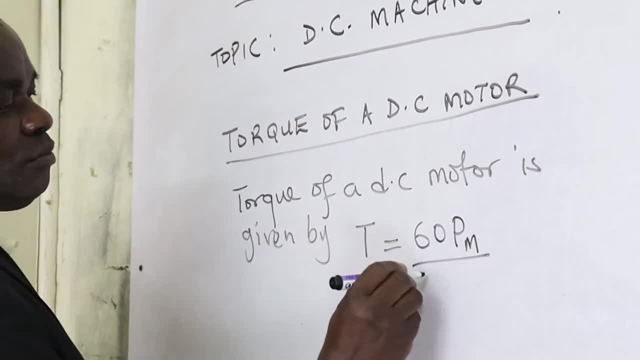 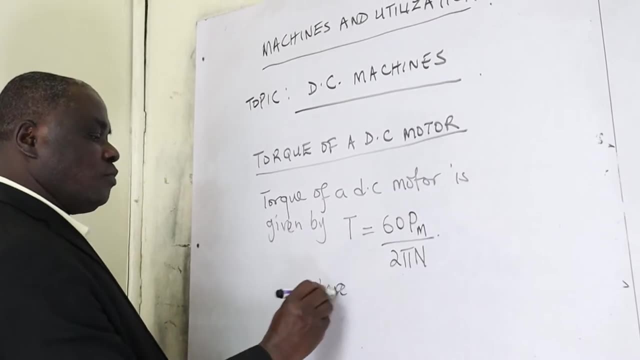 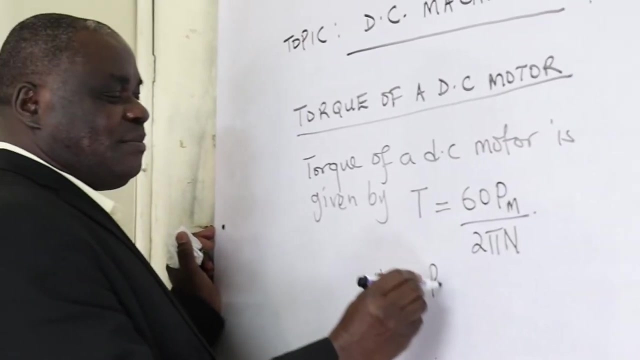 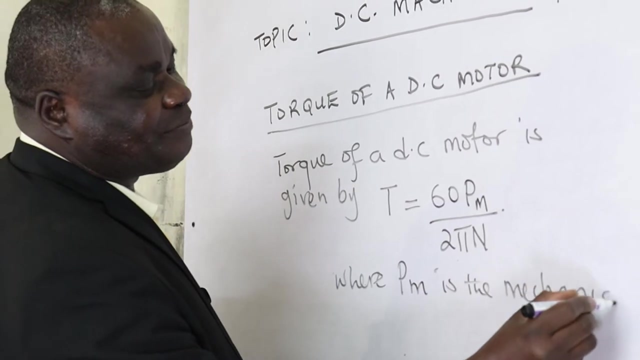 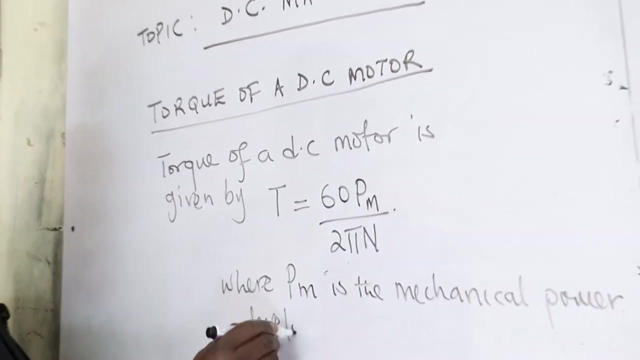 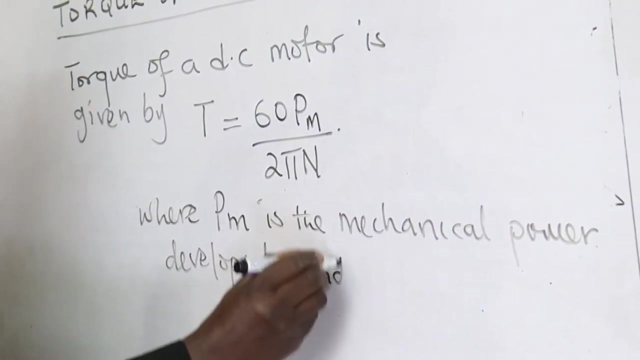 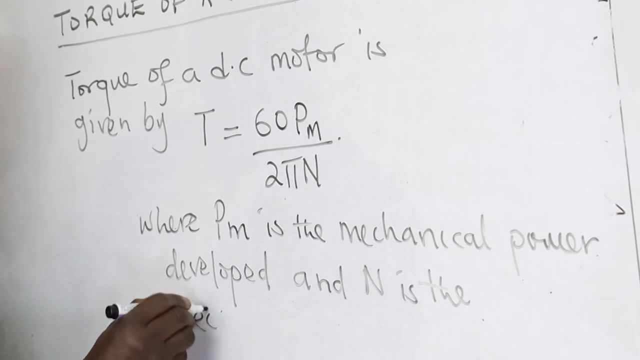 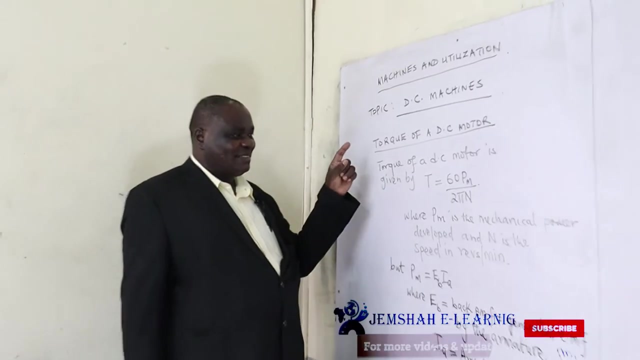 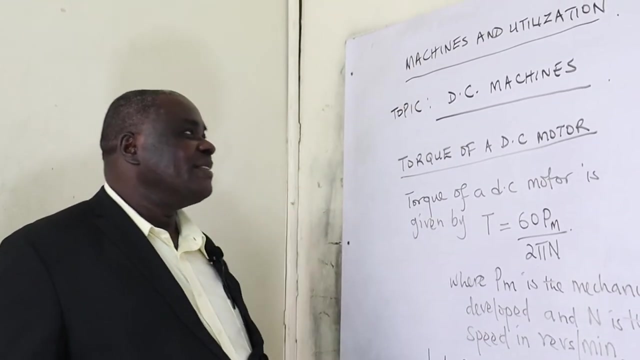 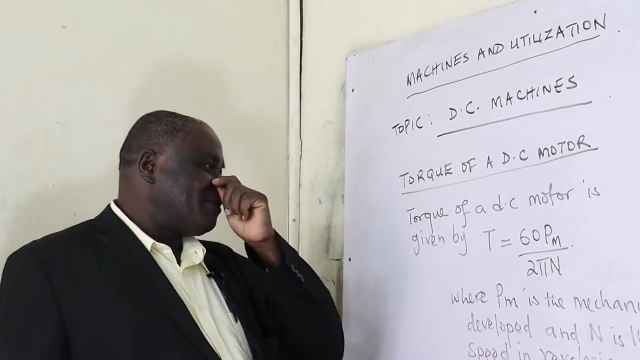 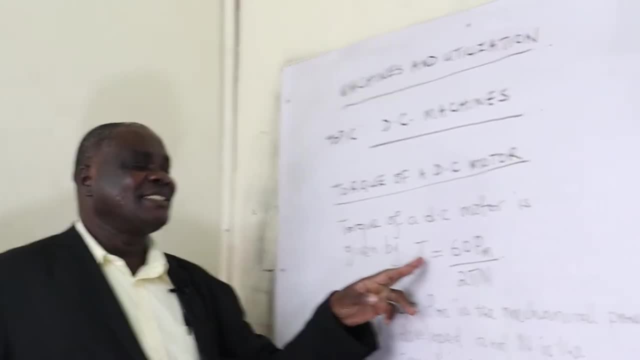 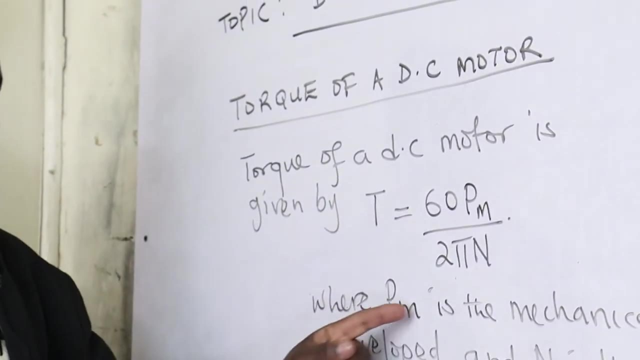 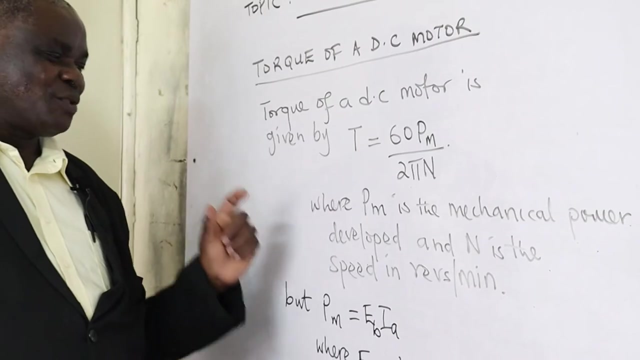 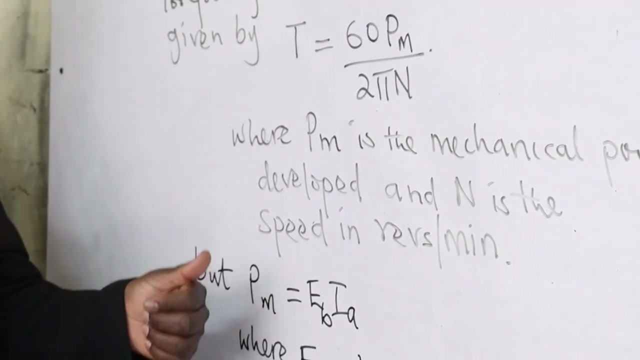 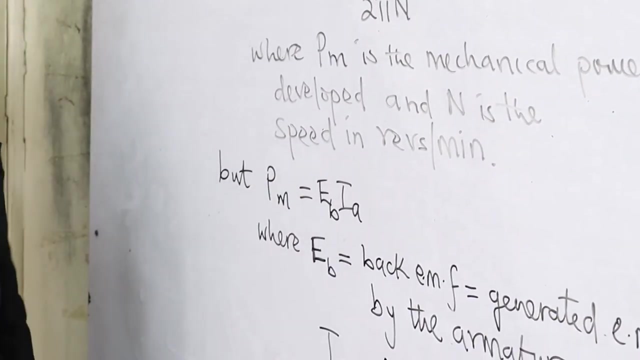 Torque over DC motor is given by T, which is equal to 60 PM, all over 2 pi N, where PM is the mechanical power developed within the armature and N is the speed in revolutions per minute. But PM can be evaluated by having back EMF multiplying armature current. 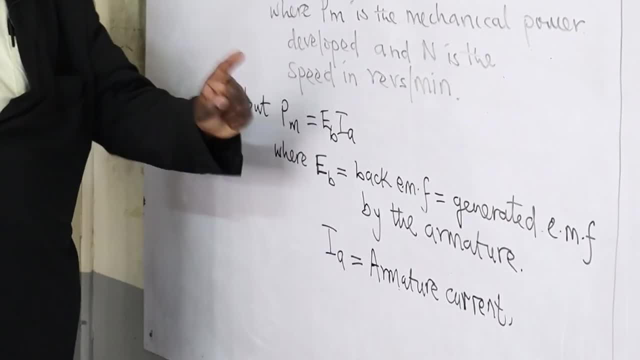 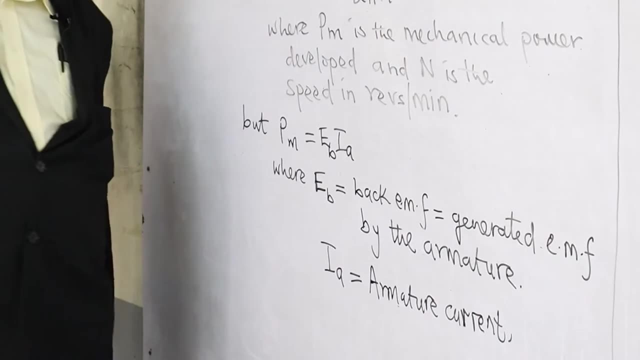 The EB is just the back EMF, which is the same as the generated EMF by the armature. IA is the armature. current EB from T is equal to 60 PM, all over 2 pi N, And it is upperכw işte conservation standard. 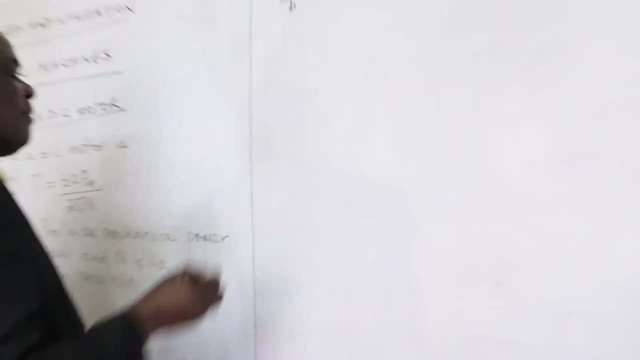 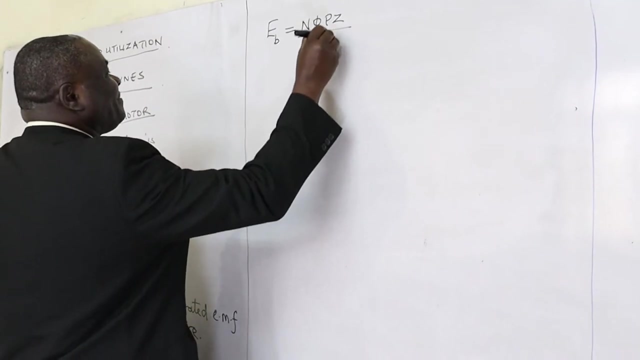 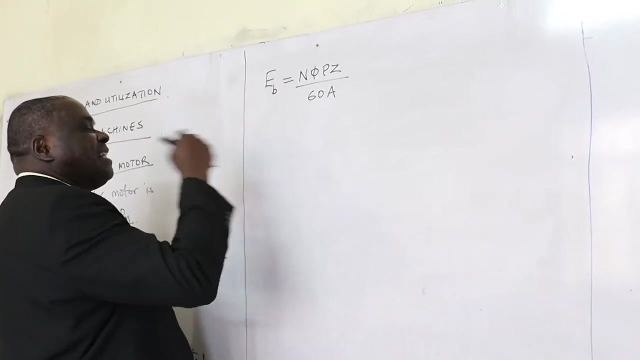 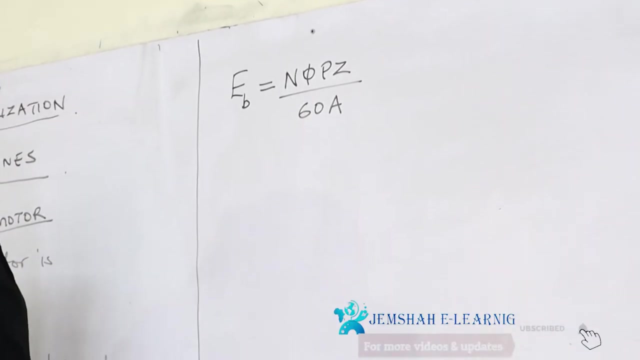 Let's see what about R. R is equal to oneąći php V, or appropriate weight of 4.. So P is the number of championship//poles within the magnetic circuit of the DC motor. Thank you, R is the…. 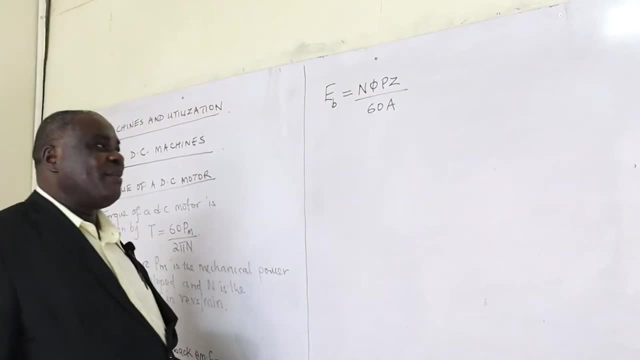 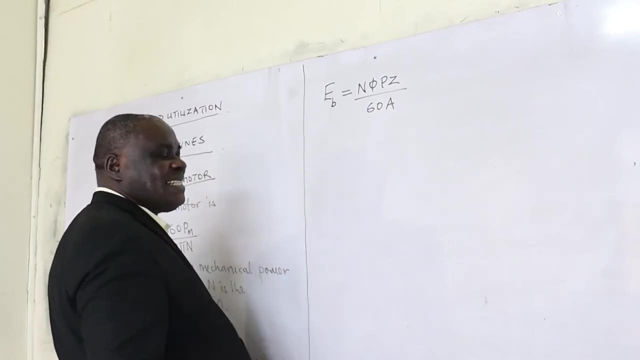 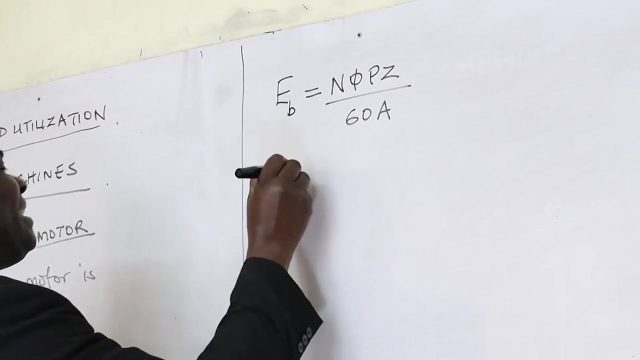 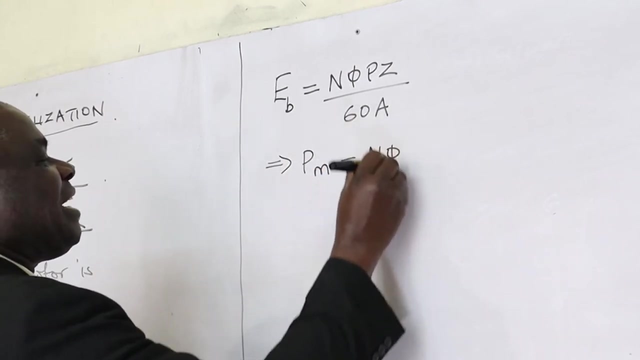 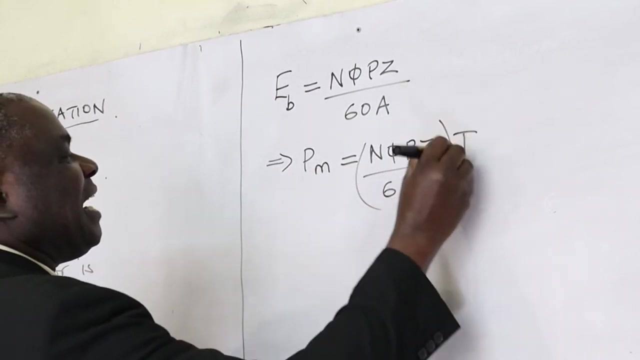 is the number of amateur conductors- number of amateur conductors- and A is the number of parallel paths within the amateur- number of parallel paths within the amateur. So this implies that our PM will be equal to NPEZ all over 60 A. now we multiply with I A. Therefore, 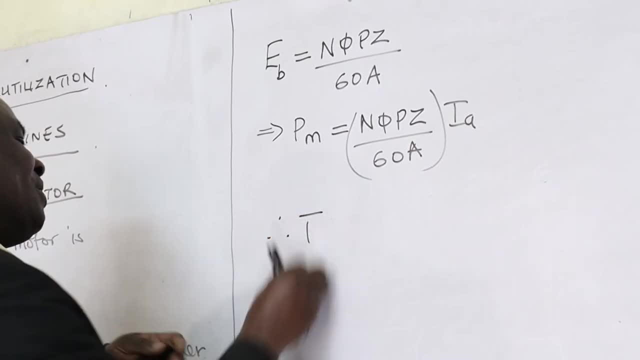 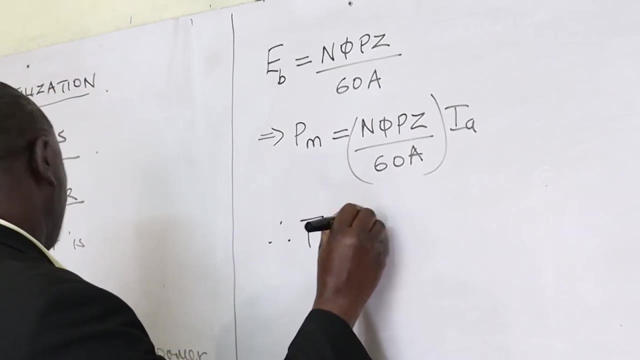 TB. t, Therefore, T which is took, therefore T which is taken is given by PM, is darbed on the pump position: savez making, Therefore, T, T, Therefore, T which is taken, therefore T which is taken, Page 4.. 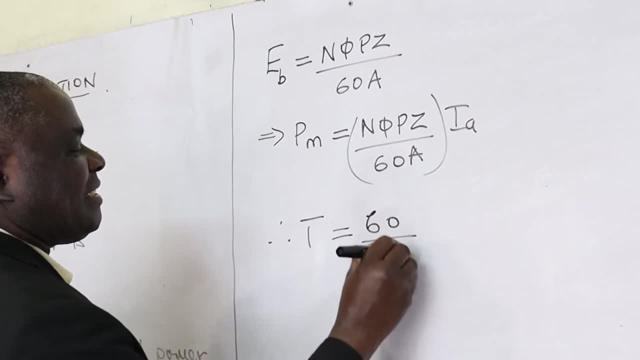 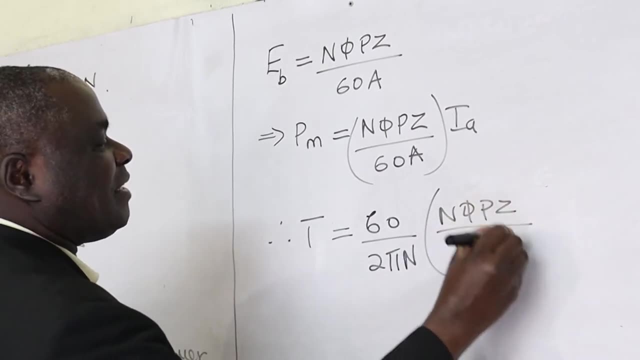 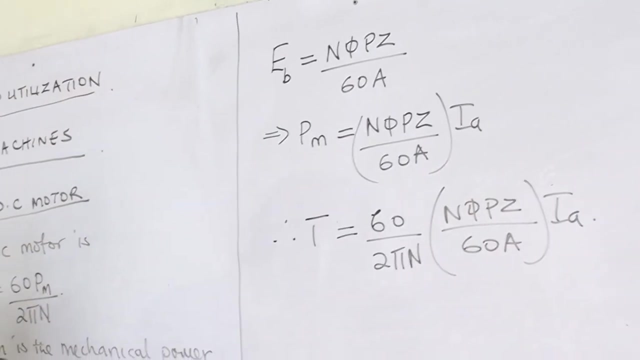 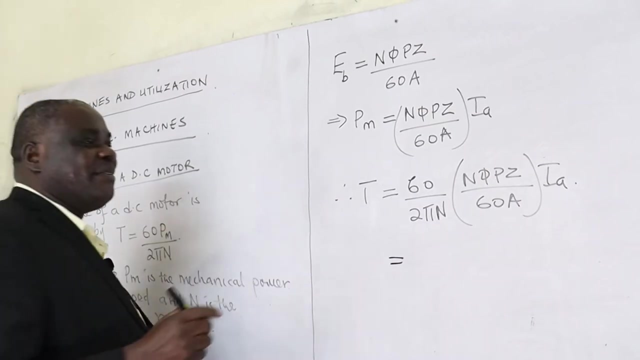 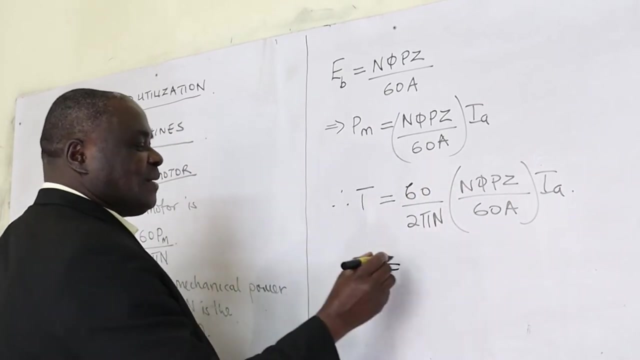 60, all over 2 pi n. now multiplying n, phi p z, all over 60 a, and all of this multiplying i a. When this one is simplified further, when this one is simplified further, this one is simplified further, we'll get this: x will cancel that 60, n and n will also cancel. 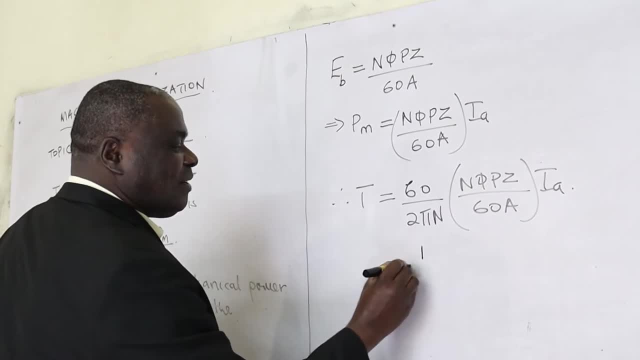 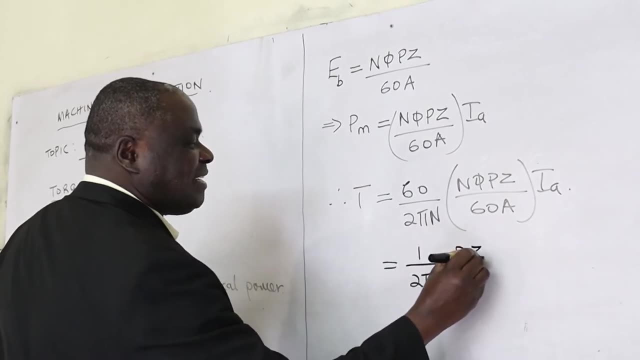 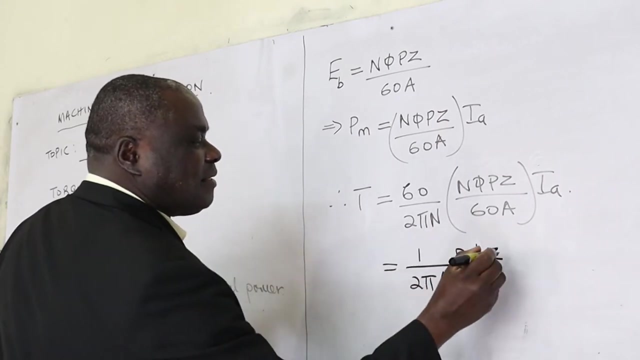 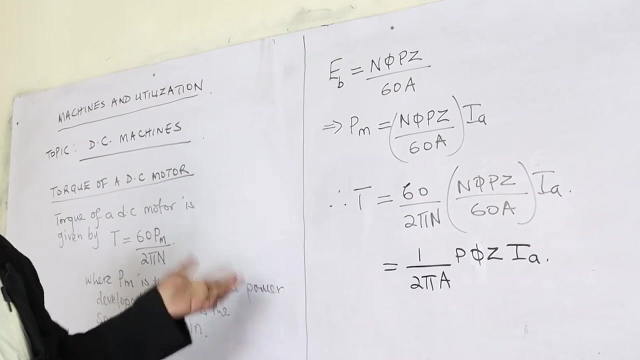 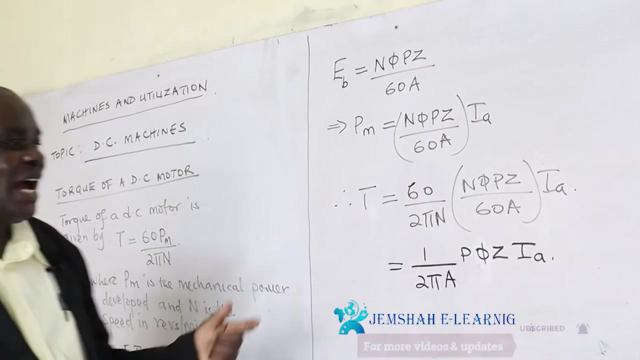 So we'll be remaining with 1 all over 2 pi a, p z, p, phi z multiplying i, a. But when a motor is already bought and it is within the premises or within where it is to be installed or already installed, you cannot be able to have p as a variable. 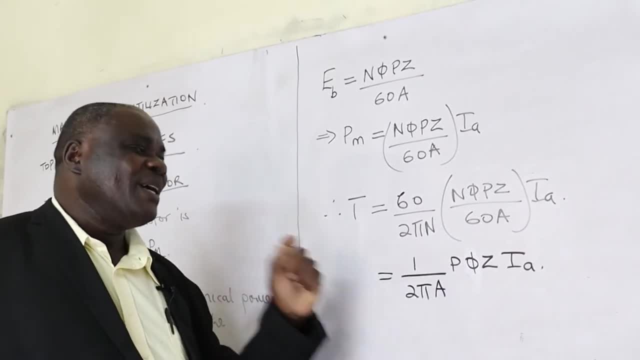 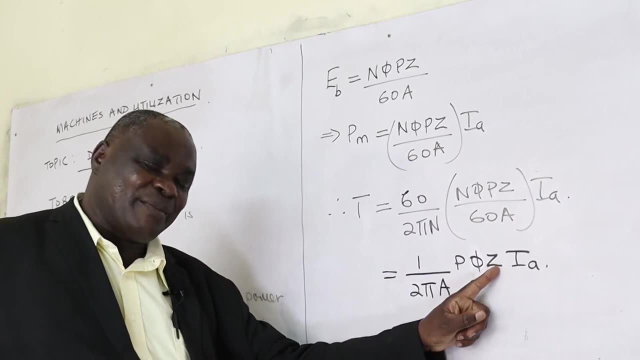 P will be a constant because the motor is already with you. there is a defined number of poles for that particular motor and we have also. you cannot change the number of parallel paths within the armature. So p and z, those ones, will be constant. 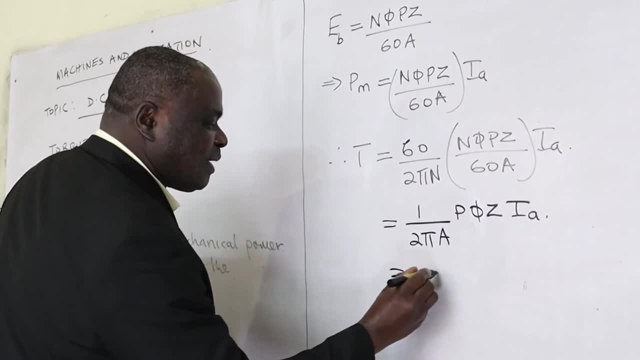 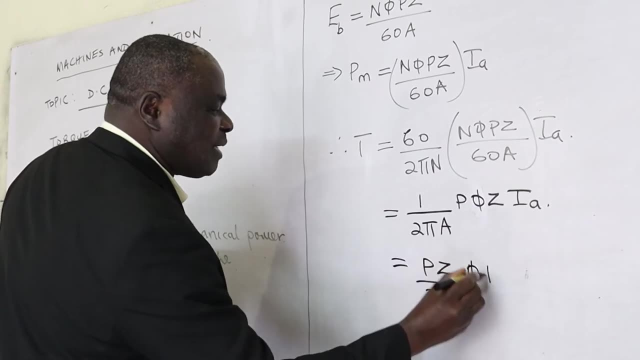 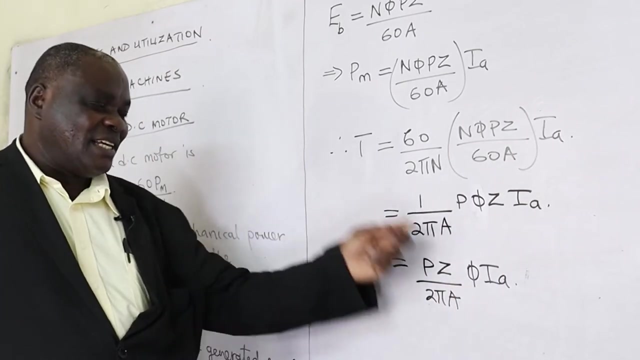 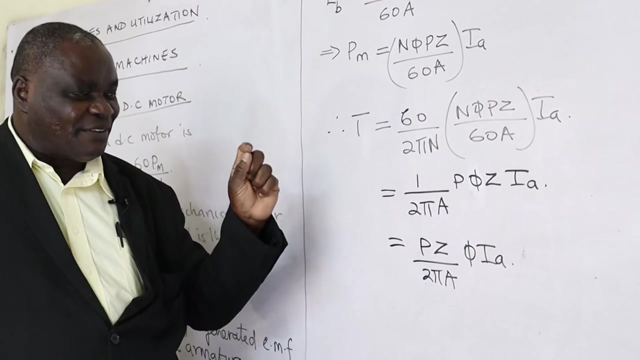 So this one will be equal to p z all over 2 pi a. Now multiplying phi, multiplying i a, Phi is the flux per pole. Now this phi is from the field circuit of that particular motor. It is the field flux for that particular field circuit of that particular motor. 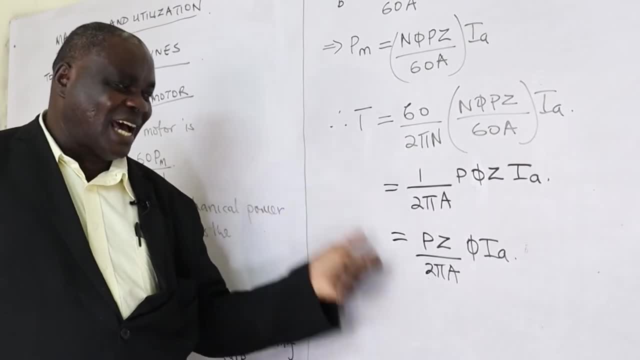 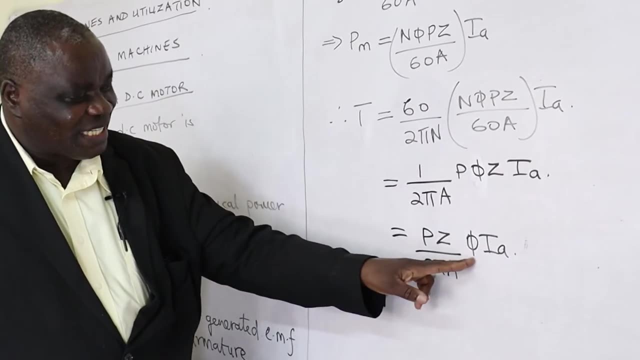 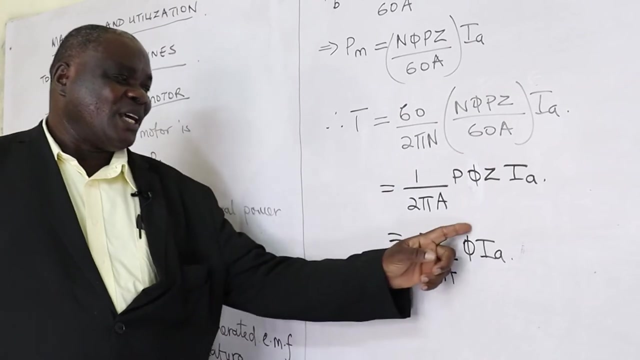 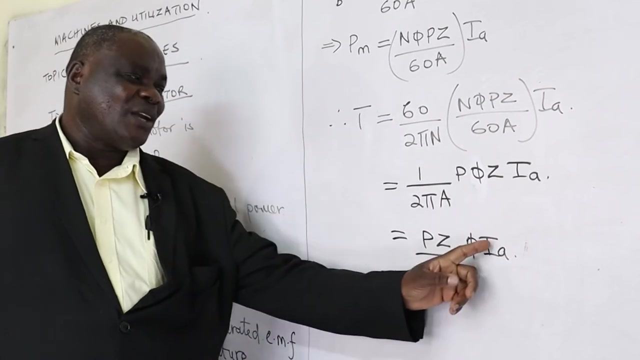 And this one can be varied depending on what is done or depending on the magnetic circuit of that particular motor. So phi can always be varied and if you verify, the torque will also vary. You can also vary the armature current, because when you have an armature circuit you can. 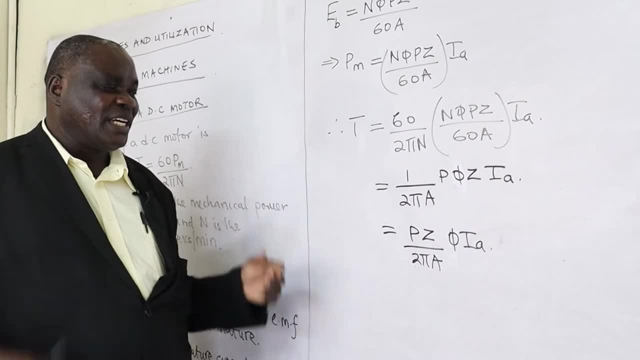 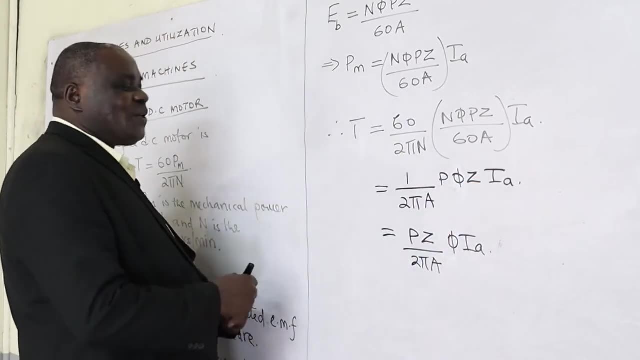 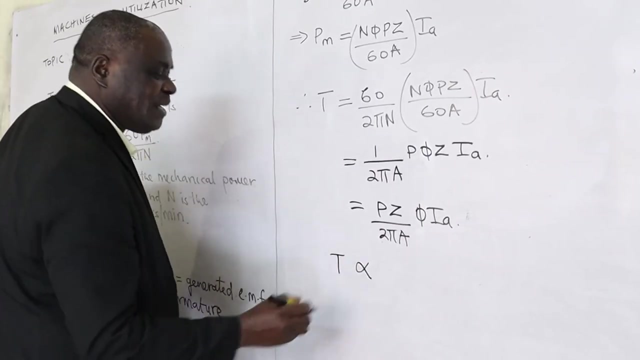 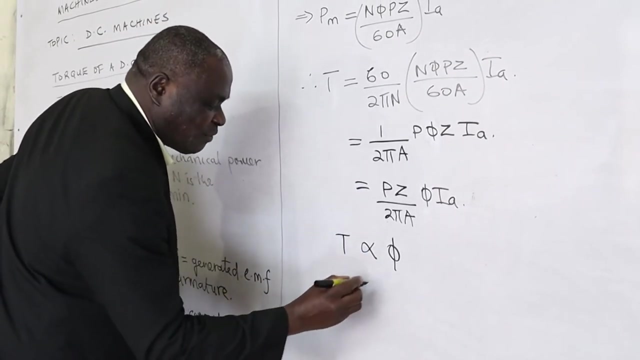 include some resistances. When you include this you can be able to vary armature current, And armature current also depends with the loading. So from this expression we can say our t is directly proportional, directly proportional to phi and directly proportional to phi i a. 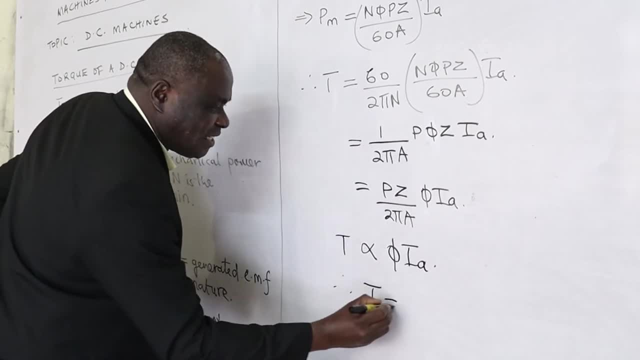 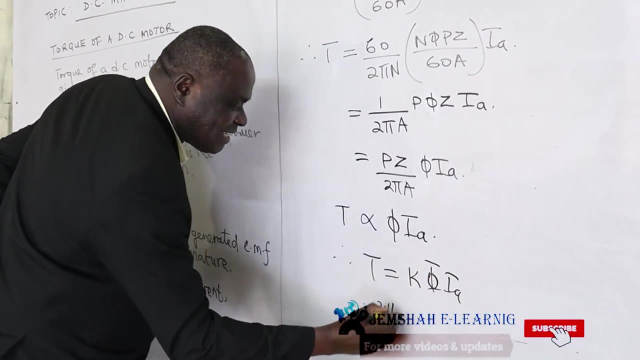 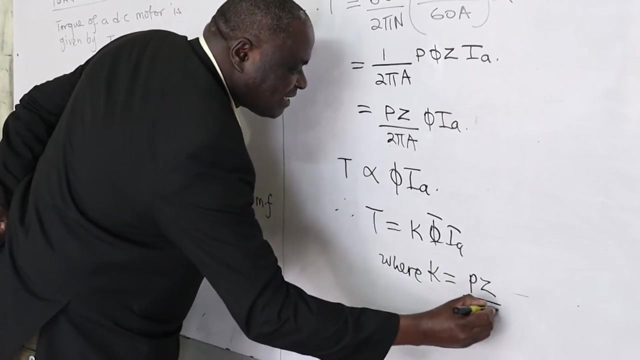 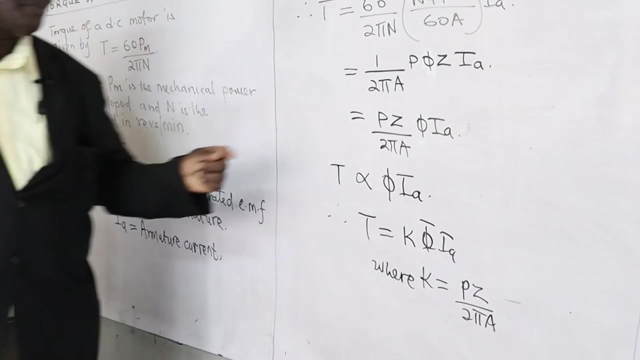 Therefore t is equal to k phi i a, where k now here is equal to p z all over 2 pi a, p z all over 2 pi a. See from this expression: when you want to increase the torque on the motor, you can. 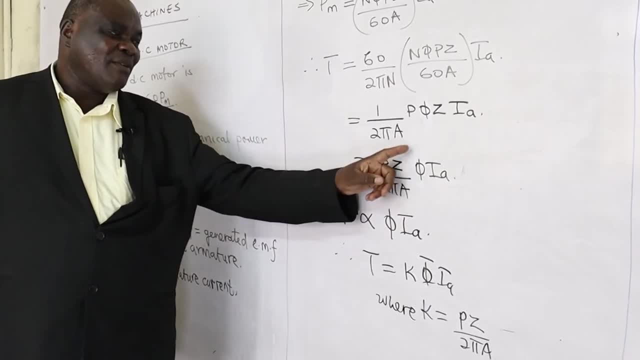 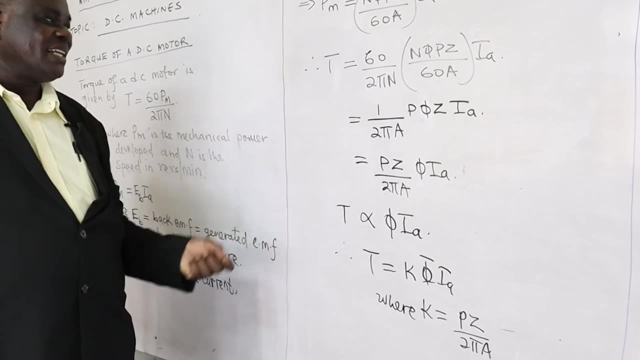 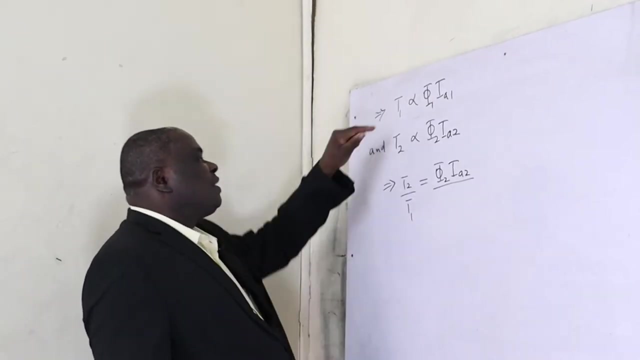 interfere. You can do something on the field flux per pole or you can do something on the armature current. When those two are varied then we can vary our torque. So t1 is proportional to phi 1 i a1.. 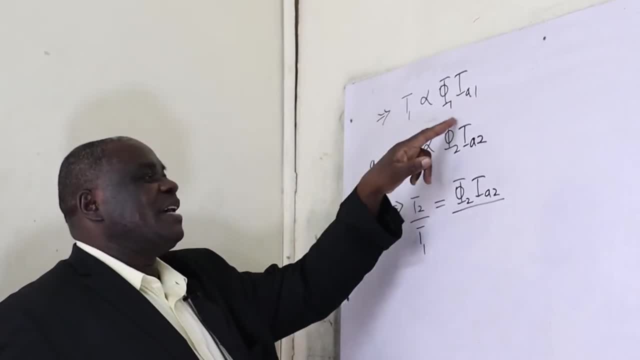 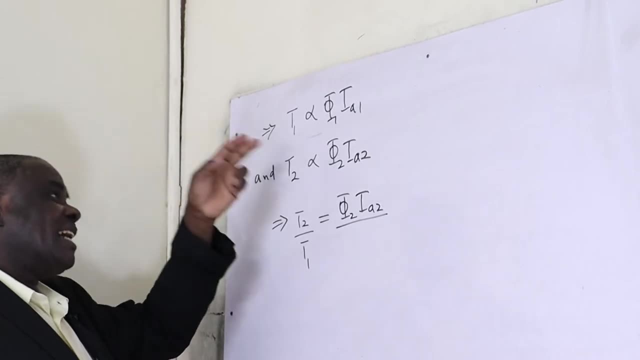 T2, that is, torque 2, will be proportional to phi 2 i a2.. So because we are working with the same motor, We have to look for the same is��. Remember it's like a back door. there are two pedals. 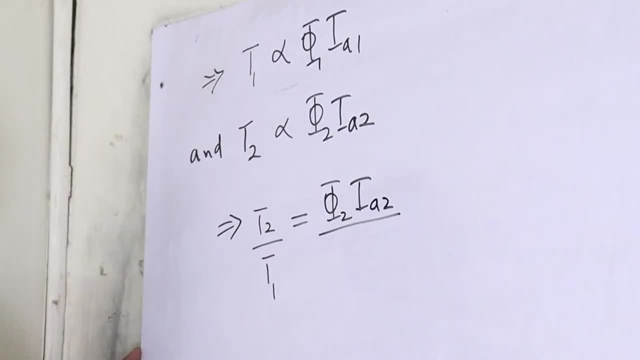 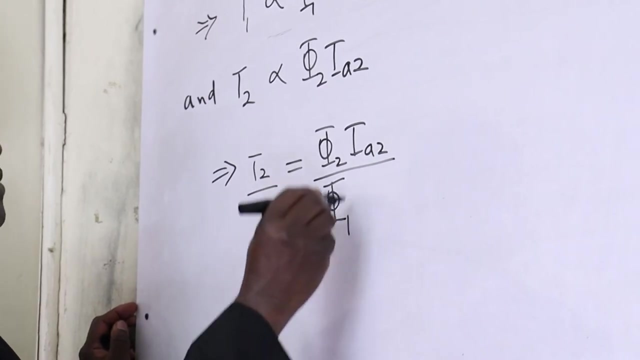 There is that constant or proportionality. So t2 divided by t1, the two constants will cancel. That is k, The two k's will cancel. We'll have t2 all over. t1 will be equal to fighter i a2, all over phi 1 i a1.. 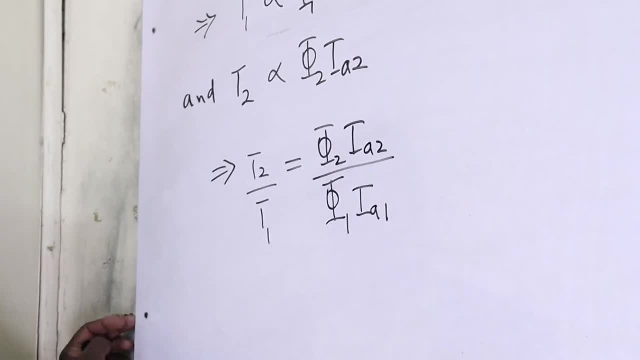 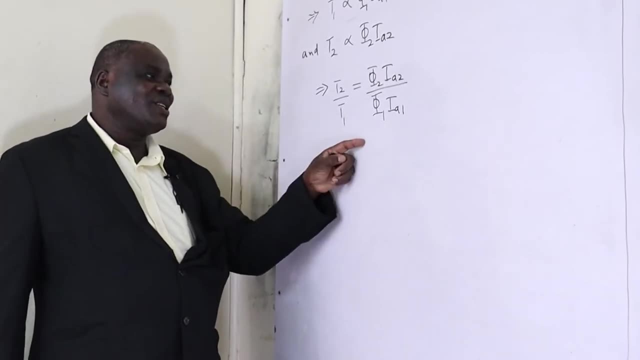 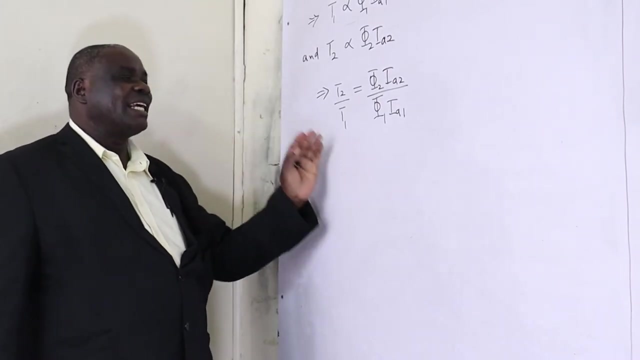 And this can be used from everything applied. Okay, chiar Lost. Uh huh, Uh huh. 07 LINCI: Uh huh, Uh huh. So T2 over t1 will cancel For analyzing the working of a DC motor under two-torque analysis. under two-torque analysis or under two-load torques. under two-load torques. 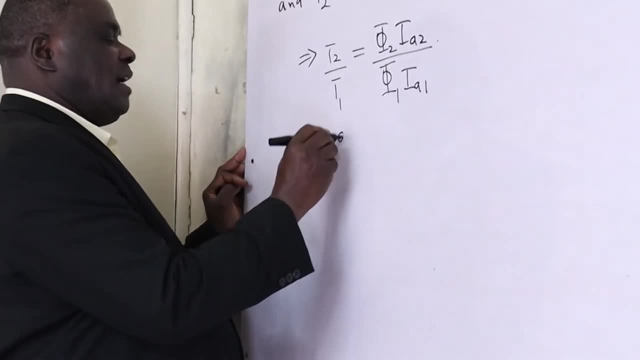 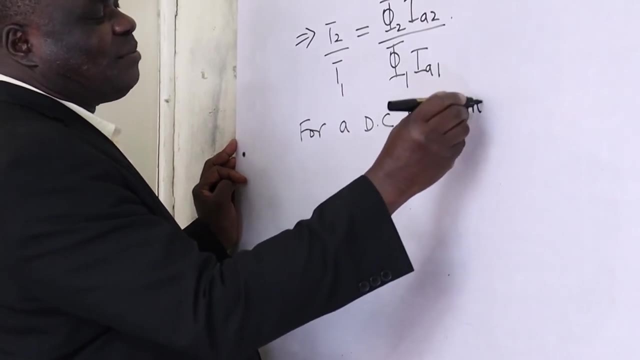 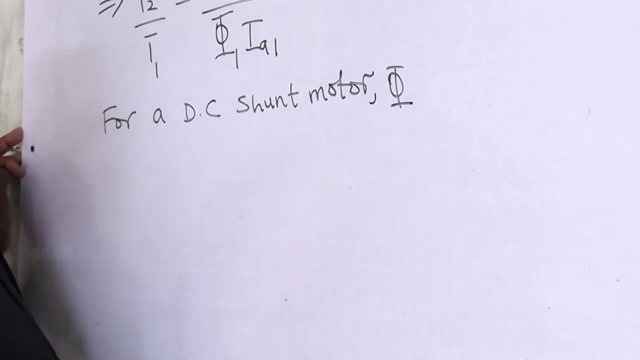 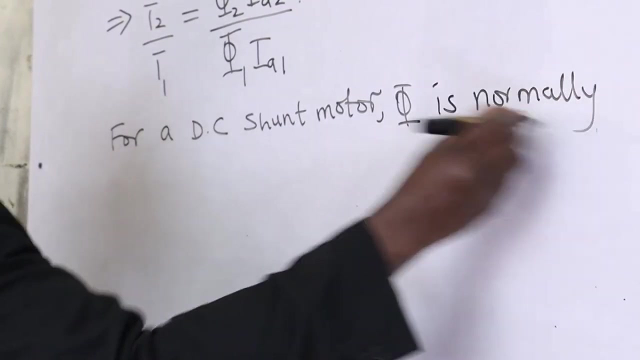 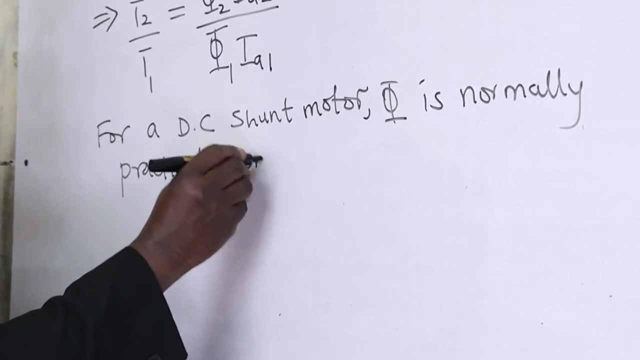 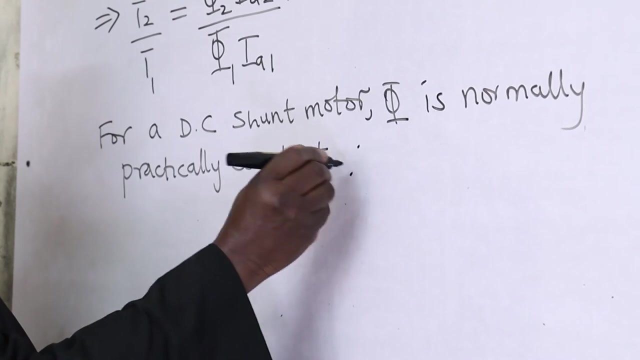 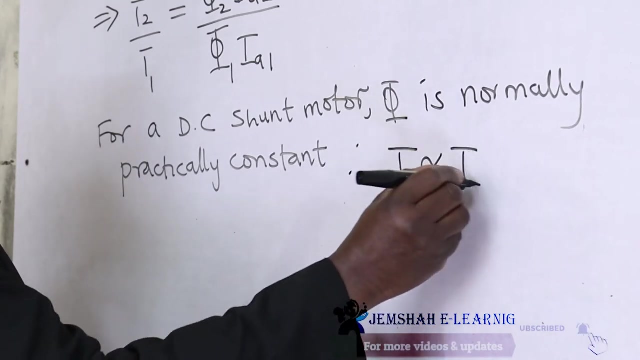 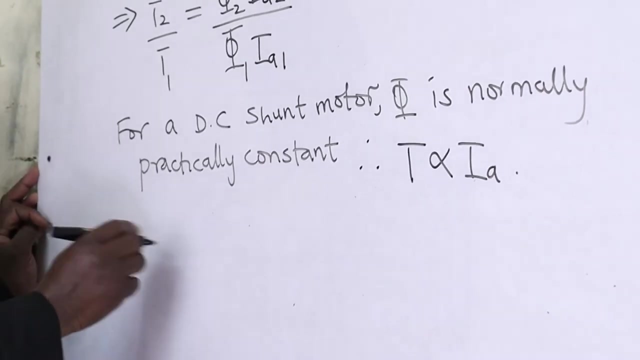 For a DC shunt motor. for a DC shunt motor, phi is normally practically constant. practically constant, It is normally practically constant. Therefore, T can be said to be proportional to IA. T can be said to be proportional to IA For a DC, for a DC series motor. 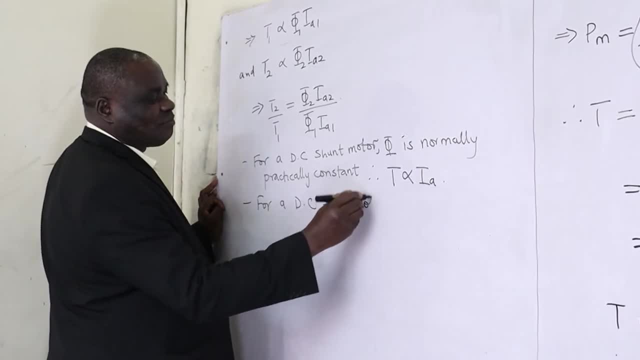 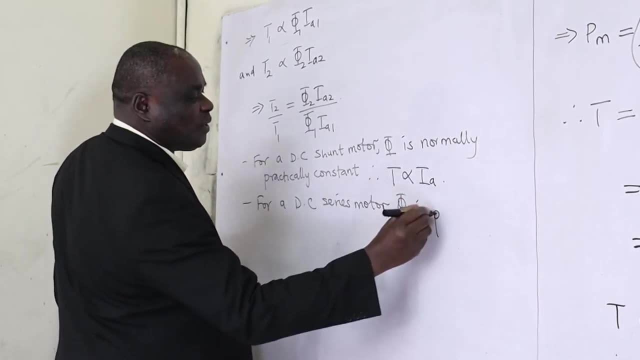 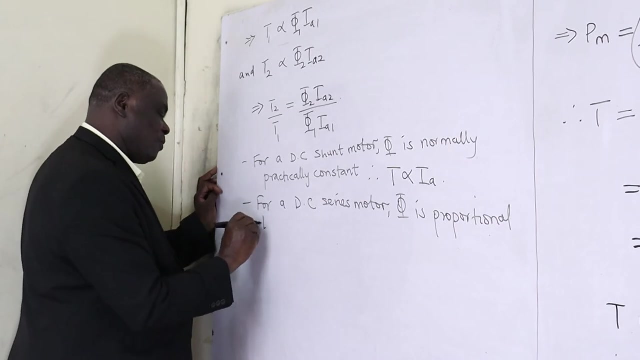 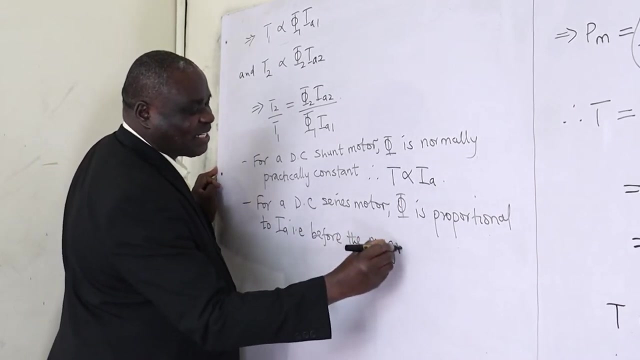 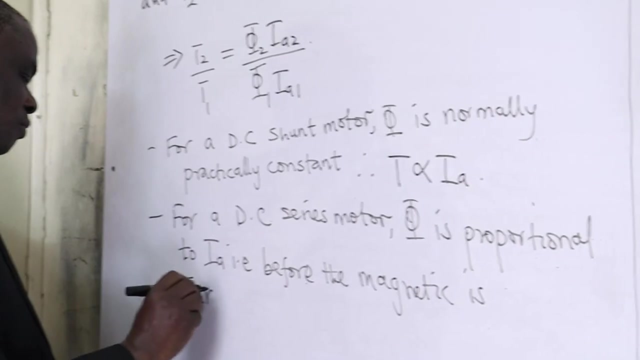 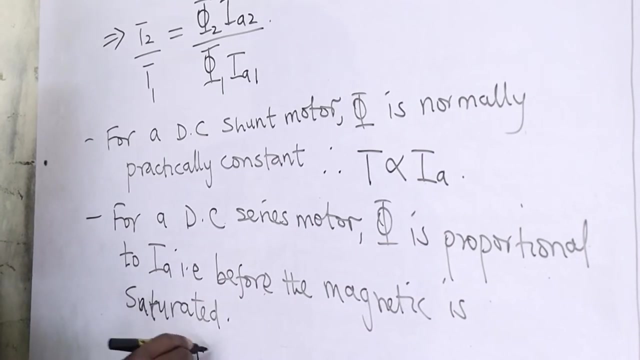 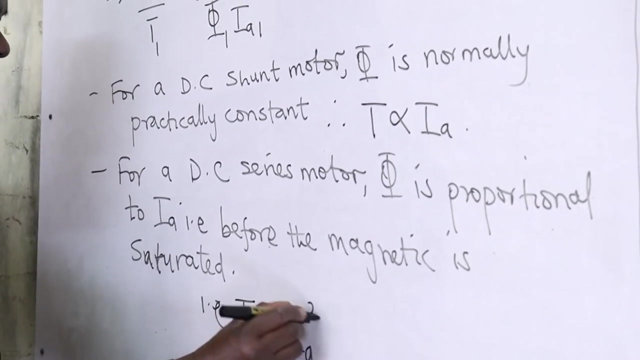 For a DC, for a DC series motor, phi is proportional. phi is proportional to Ia, that is before the magnetic circuit is saturated. that is before the magnetic circuit is saturated, That is, T will now be proportional to Ia squared, that is, T will be proportional to Ia squared. 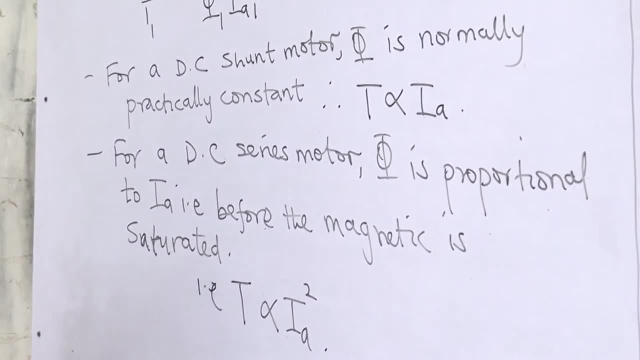 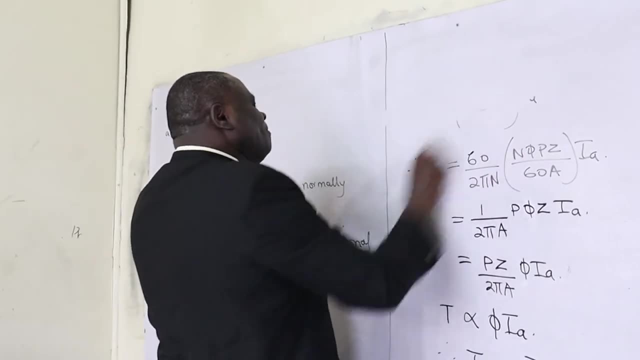 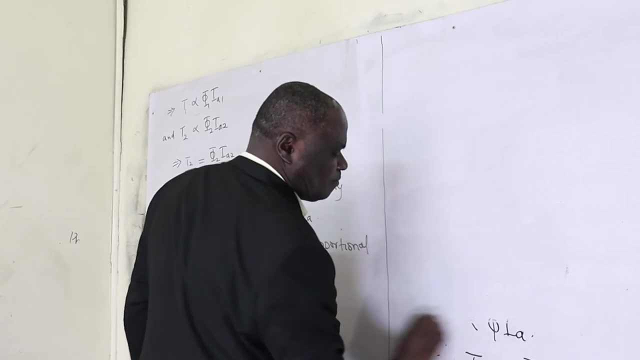 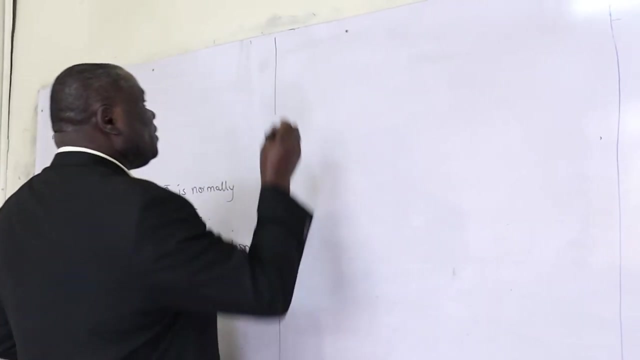 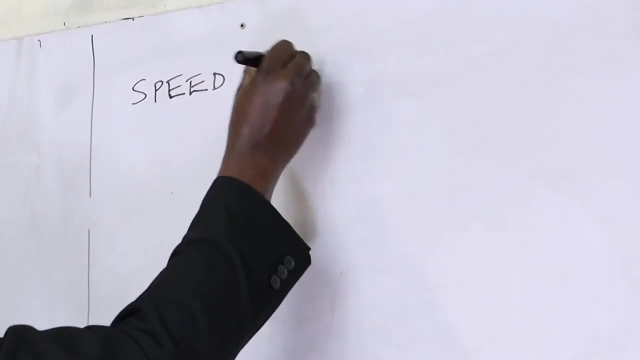 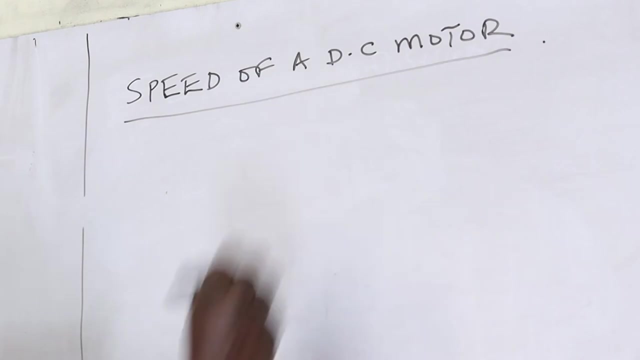 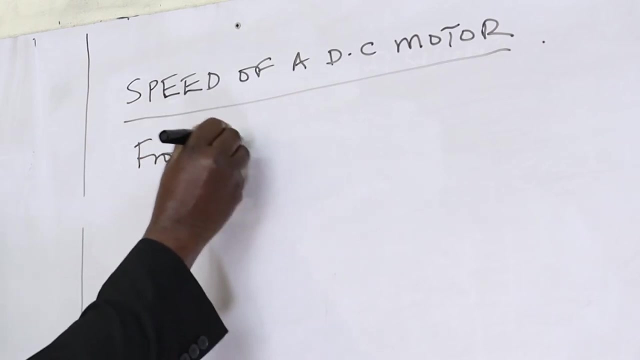 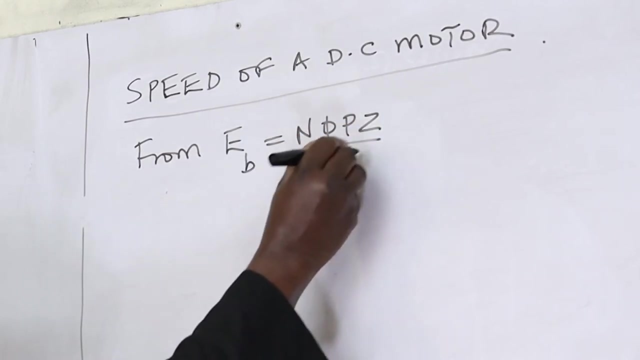 Speed already implemented. Speed already. Speed already, Anymore, of a DC motor. Speed of a DC motor From AB equals to N5 PZ, all over 60A. from this we can make N the subject, because N is the speed of the motor. 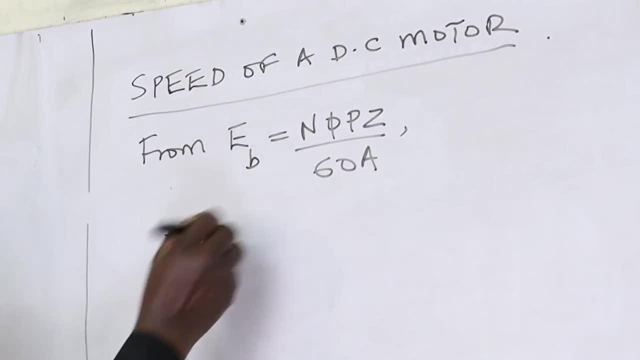 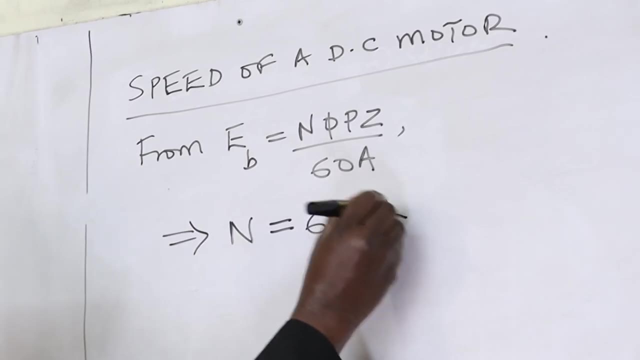 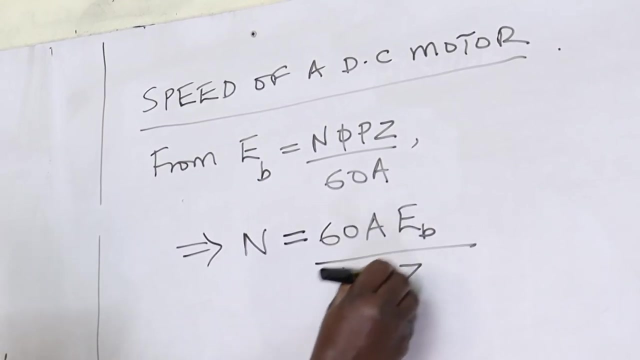 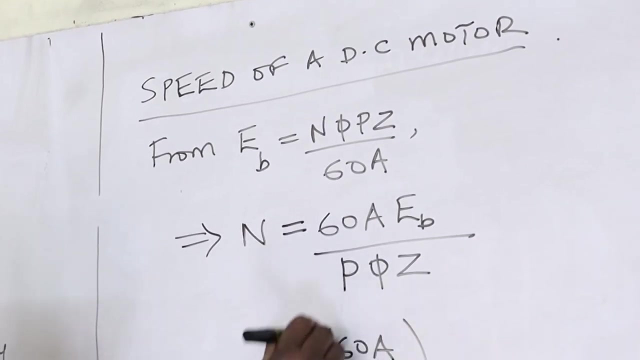 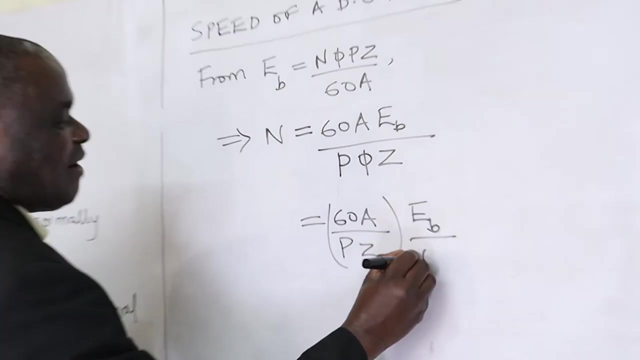 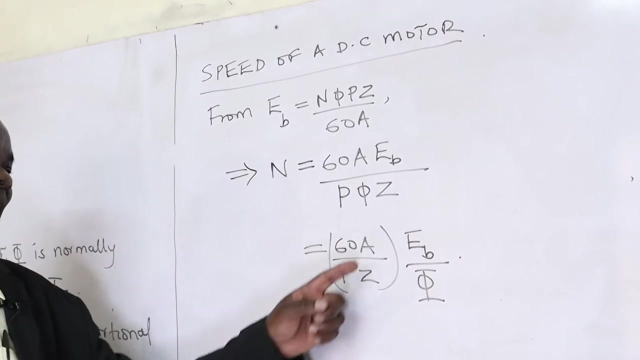 This implies N is equals to 60A. multiplying AB all over P, PZ. 60A all over PZ. the whole of this is a constant. now, multiplying AB all over 5. multiplying AB all over 5. now, 60A all over PZ. 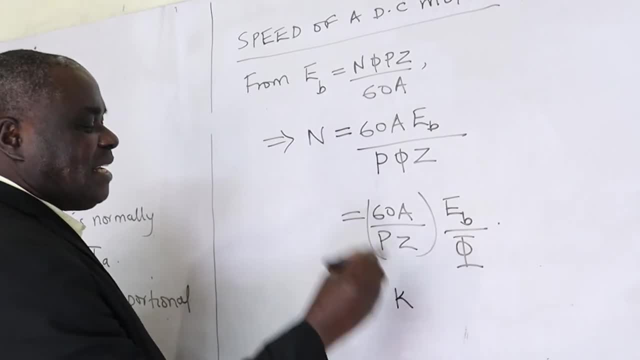 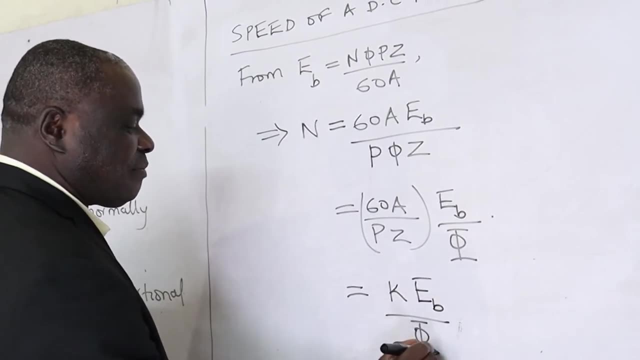 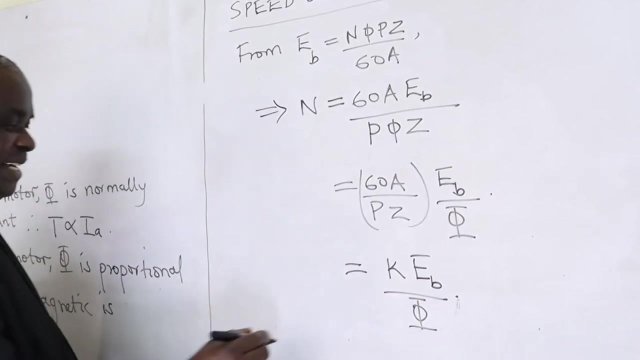 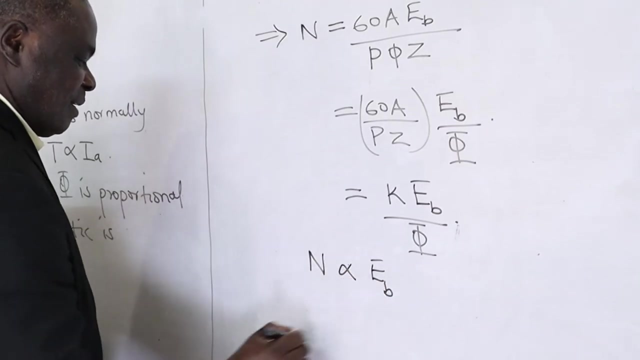 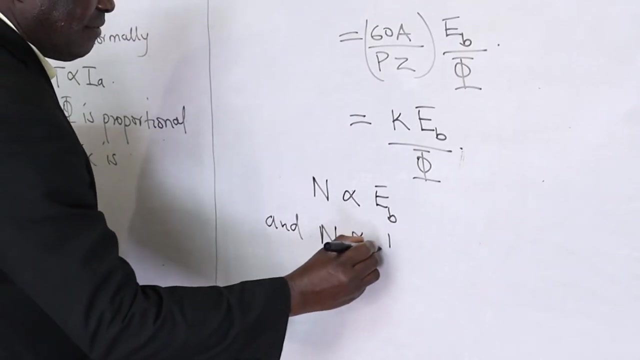 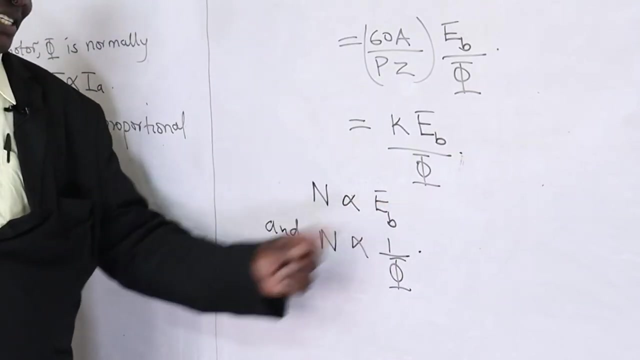 is a constant, so we can replace it by, let's say, a constant K multiplying AB all over 5. from this expression we can see everyone that speed N is proportional to AB and N and N is inversely proportional to the field flux. so when you increase AB, 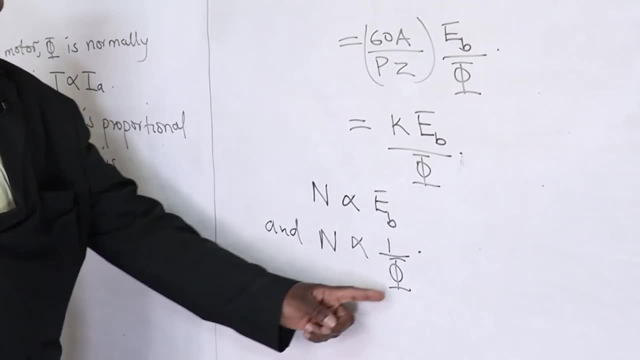 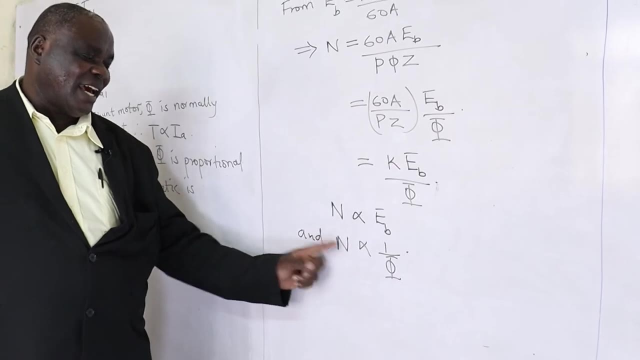 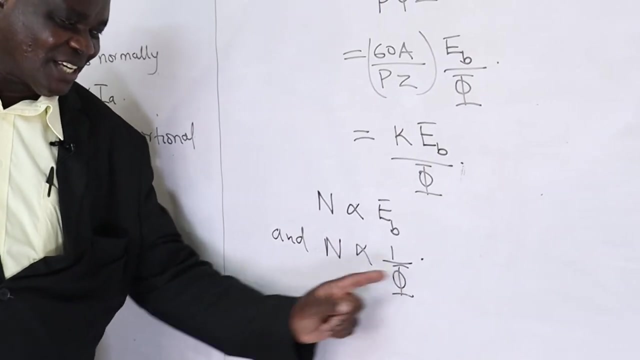 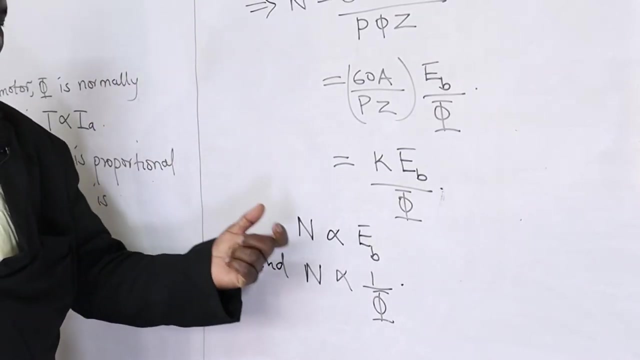 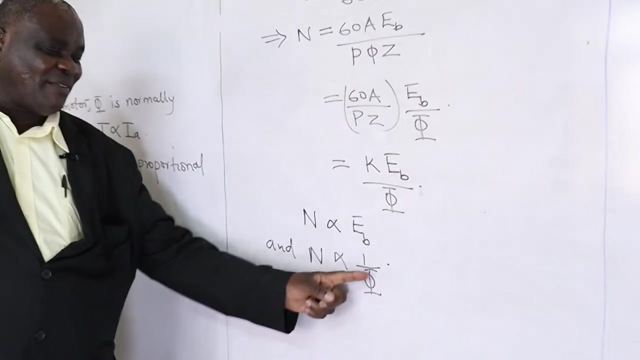 N will be decreased. when you increase field flux, N will be reduced. when you decrease field flux, N will increase. but the increase in N by the reduction of field flux cannot proceed until we check on the amateur reaction. because if you decrease the value of the field flux, such that the effect of the amateur reaction becomes critical, then the motor will not now operate. therefore, reduction of reduction of field flux while trying to control the speed of LDC motor should also be done as we check on the amateur reaction of field flux of field flux. 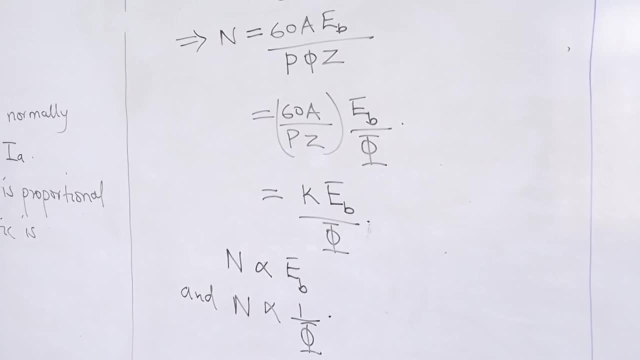 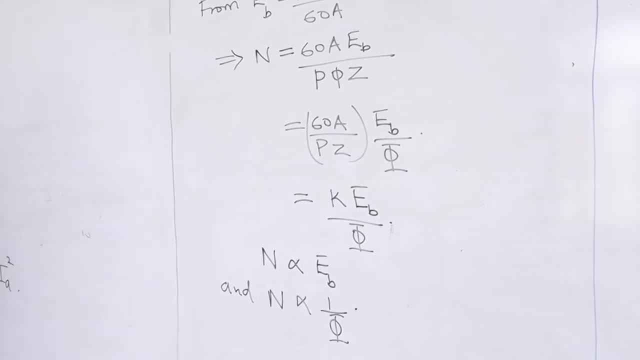 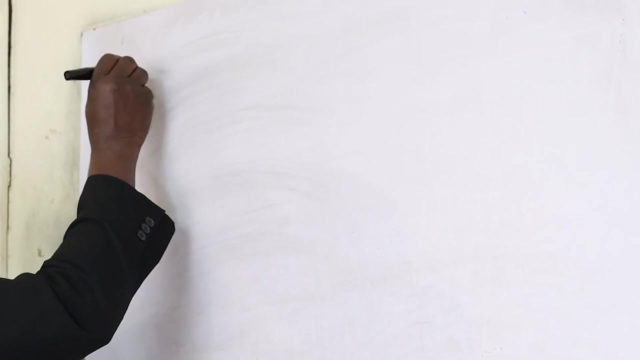 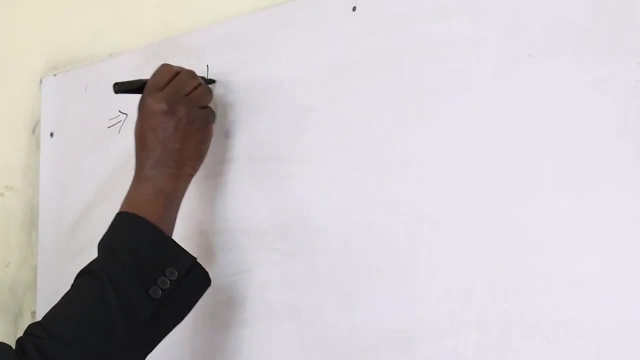 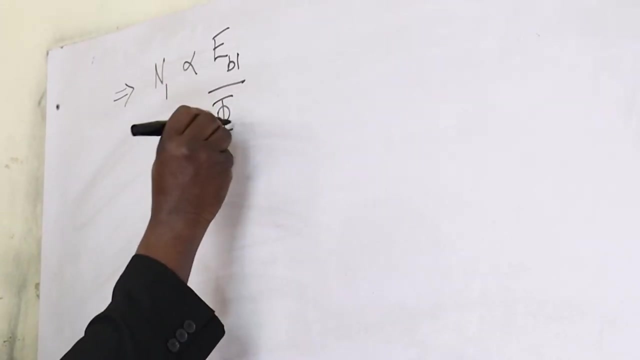 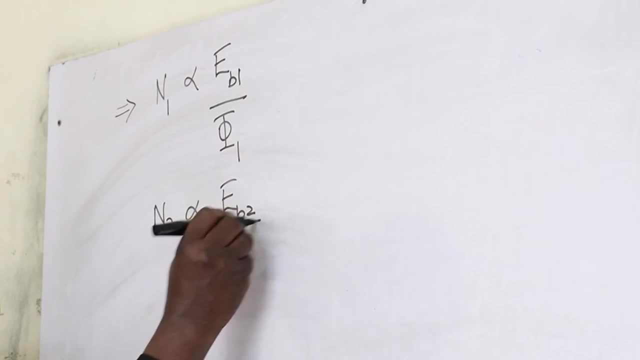 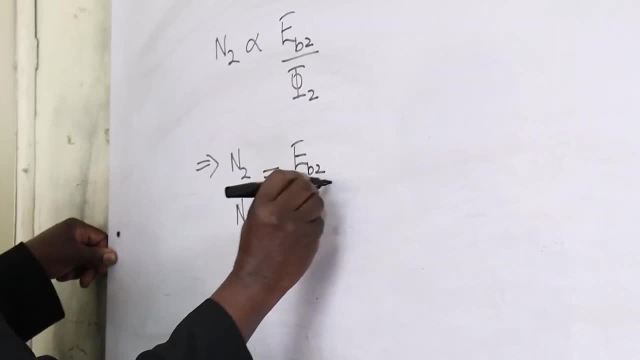 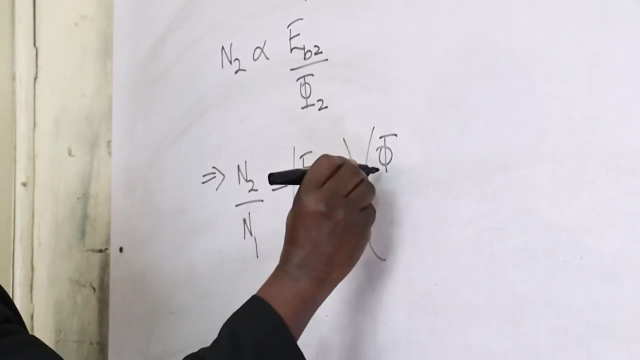 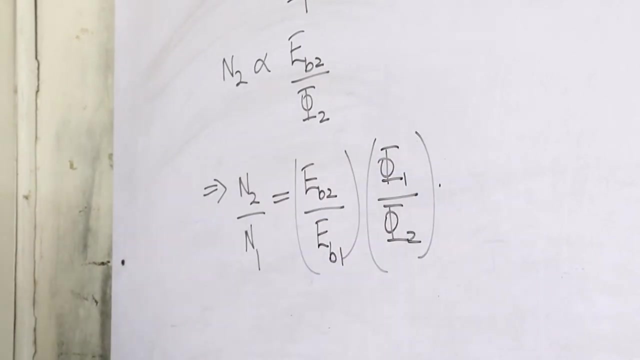 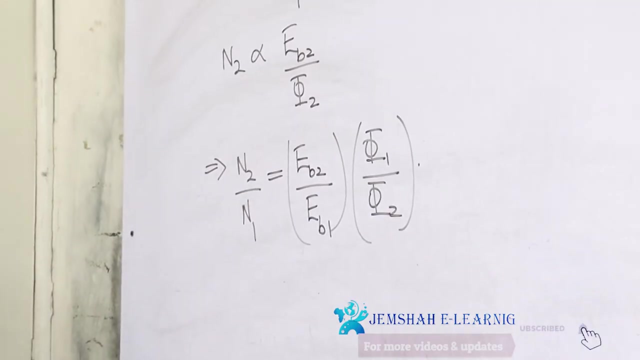 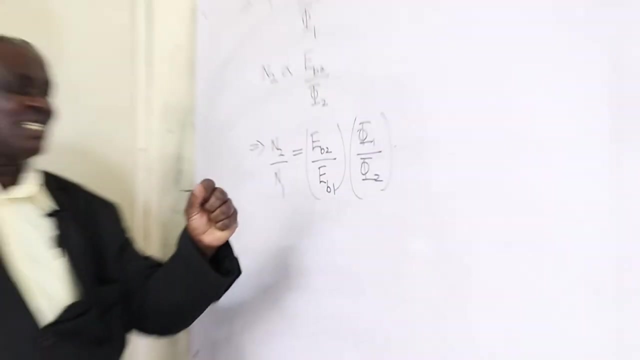 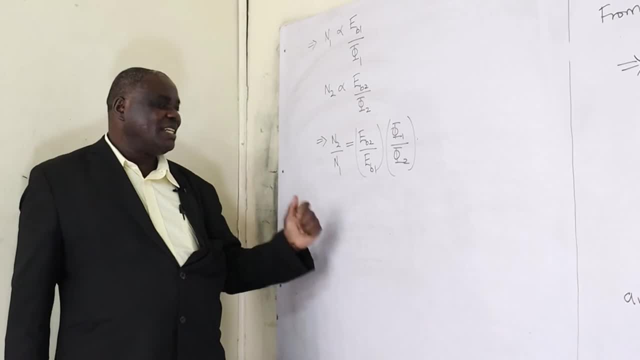 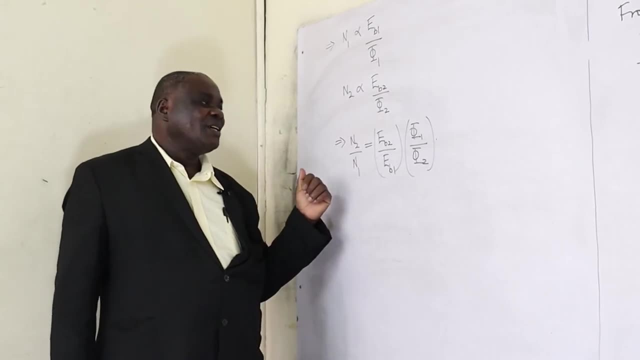 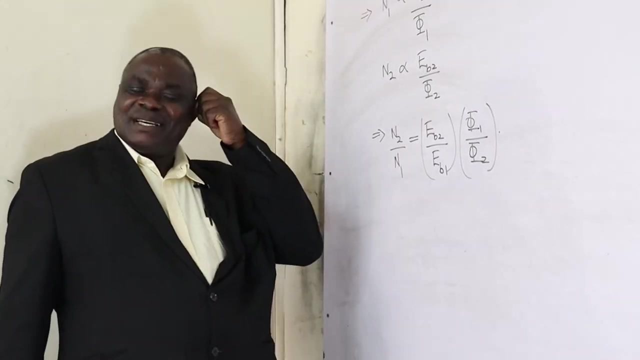 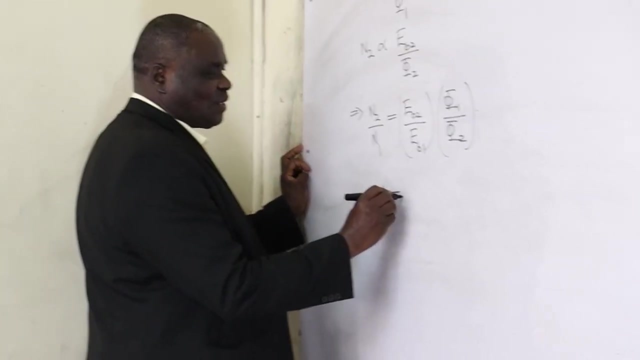 analysis of the speed when analyzing the speed of LDC motor. so there are instances you would like to increase the speed, so you must know what will happen to the field flux, what will happen on the back EMF. so from the equation N is equal to from the equation. 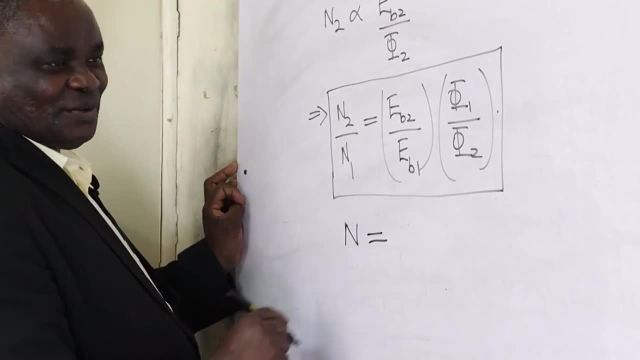 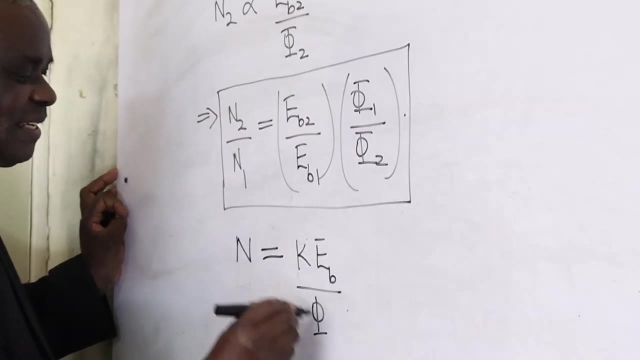 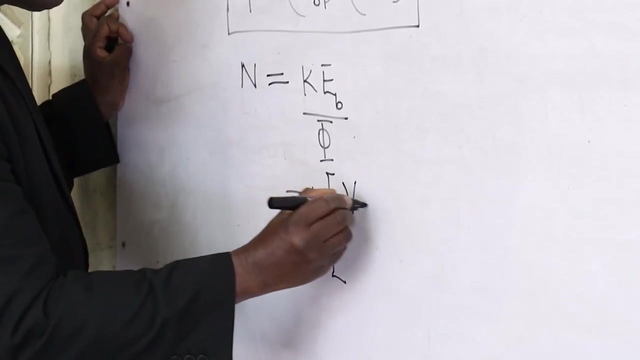 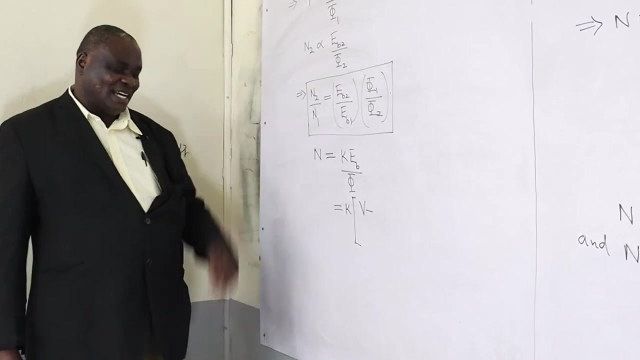 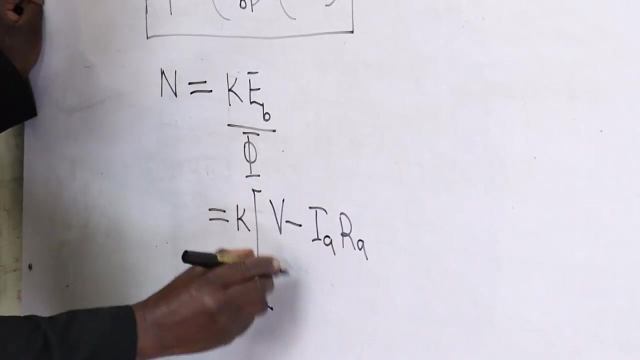 from the equation, N is equal to K to EB, all over phi, which will be the same as K into EB, can be found, taking a case of, let's say, analysis of the most common DC motor, the shunt motor. so V minus IA RA will give us EB. 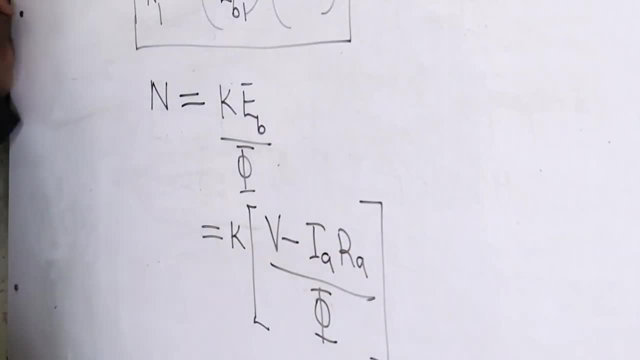 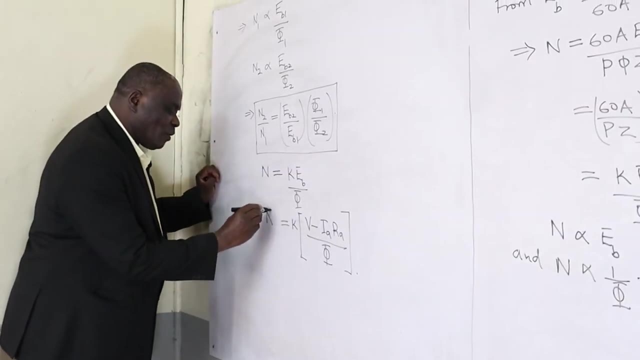 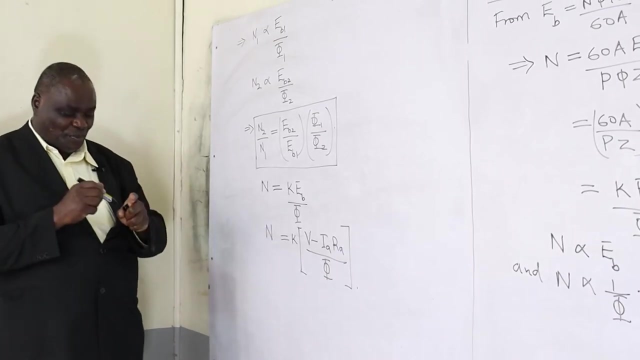 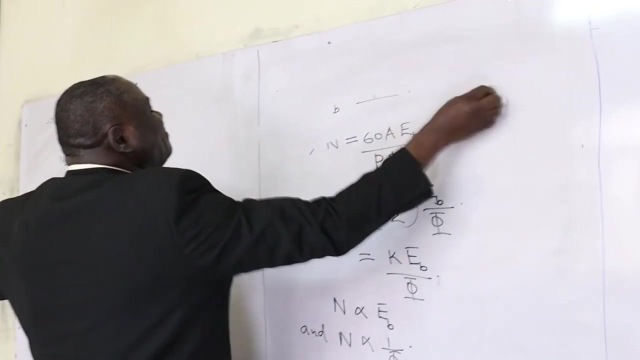 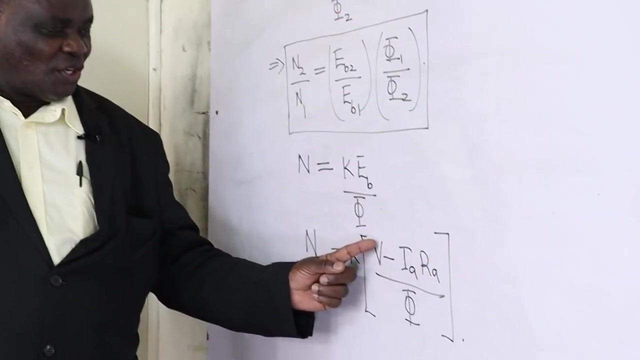 all over phi. so from this expression, so from this expression, we could deduce, we could deduce three methods of controlling the speed of a DC motor, three methods of controlling the speed of a DC motor. so check on this now. if we V is here, that is the voltage. 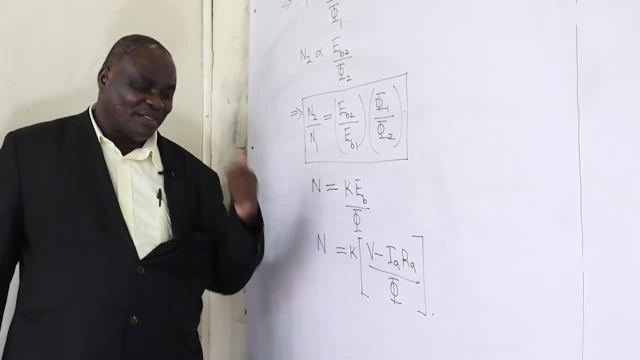 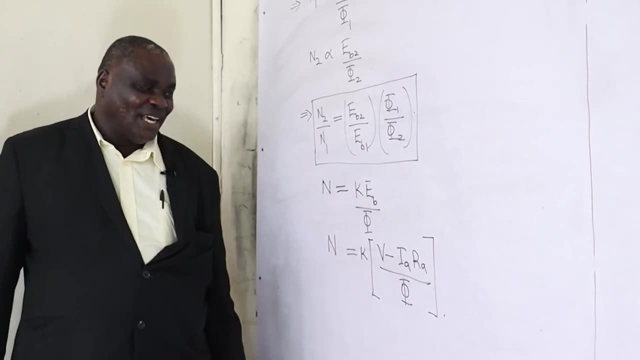 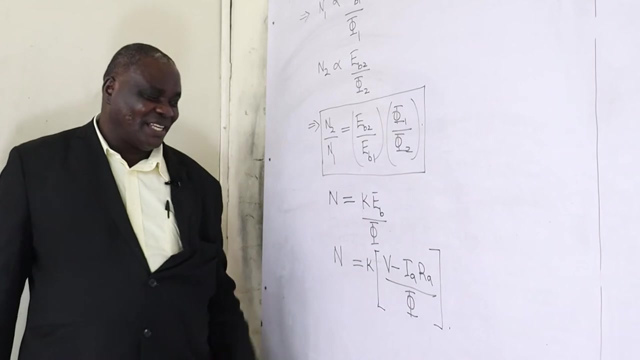 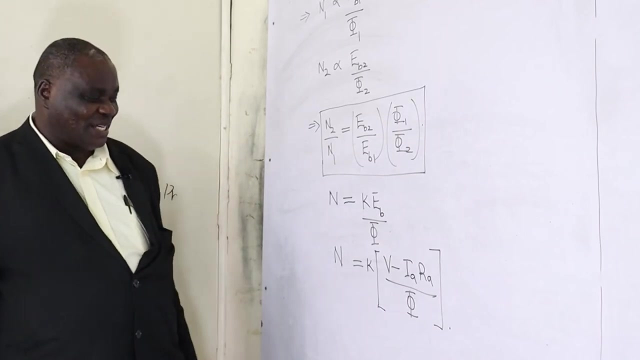 input voltage to our motor. if you do something on the input voltage, if you try to vary that one, it will give you a change in speed. if you do something to the armature circuit, then there will also be a change in speed. if you do something on field flux, 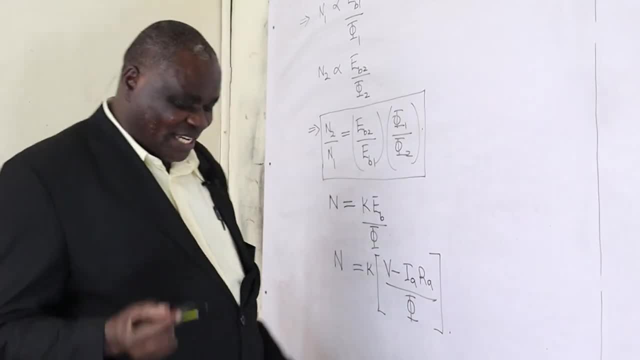 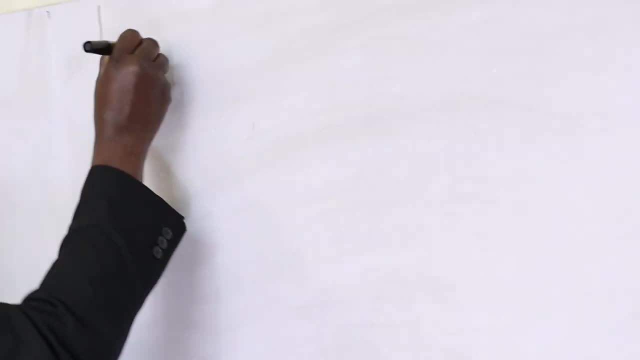 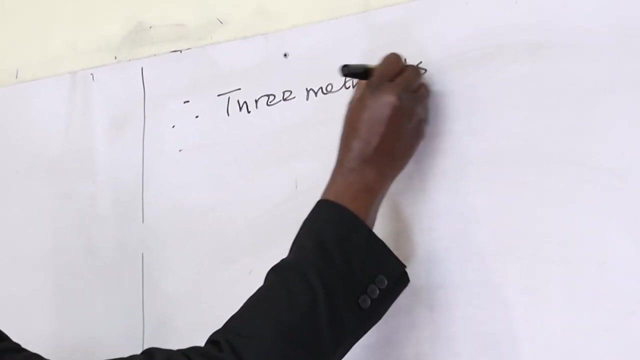 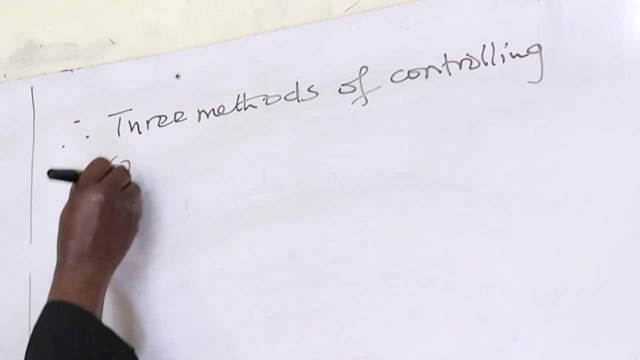 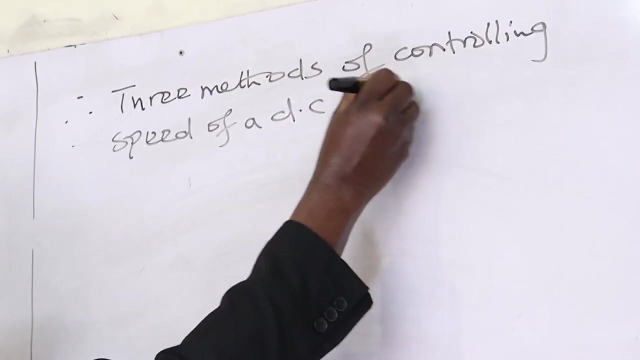 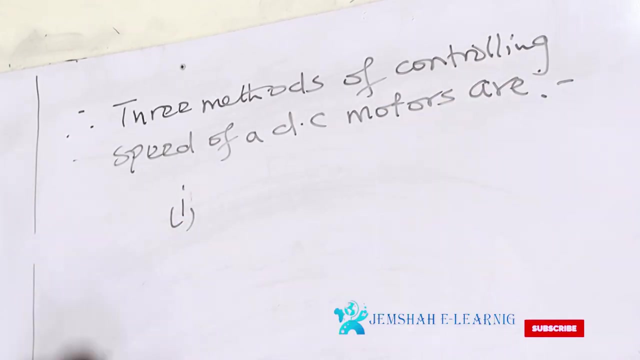 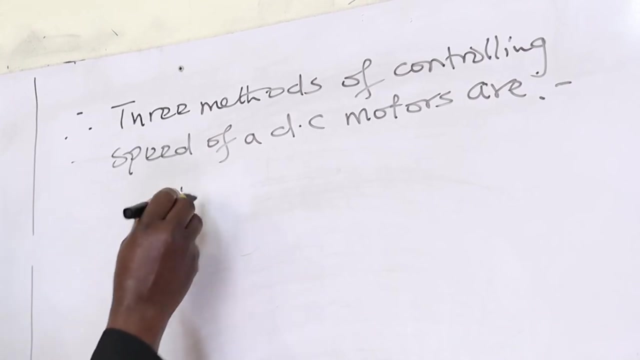 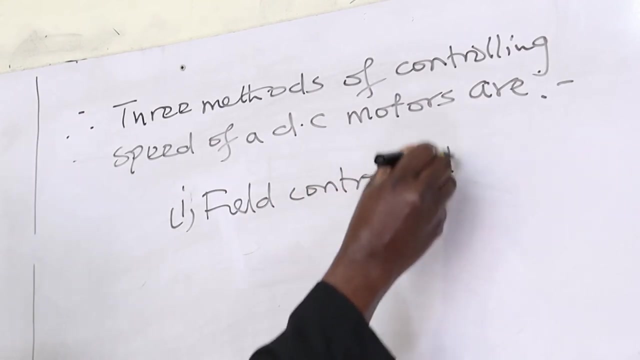 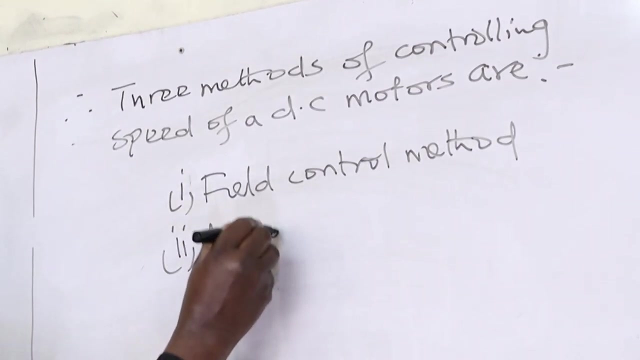 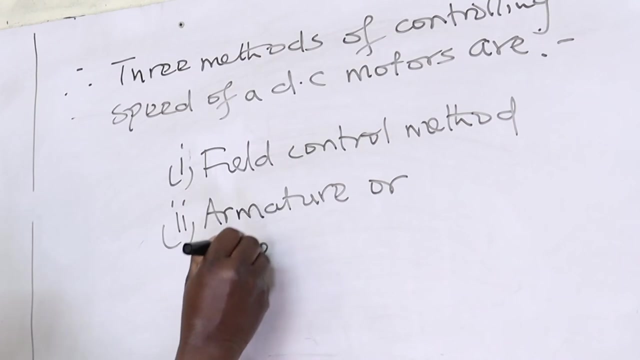 this brings to us three methods of controlling the speed of a DC motor. therefore, three methods, three methods of controlling the speed of a DC motor. they are r? r one and field control metal and field control metal. Amatya, Amatya, Aurea, static. 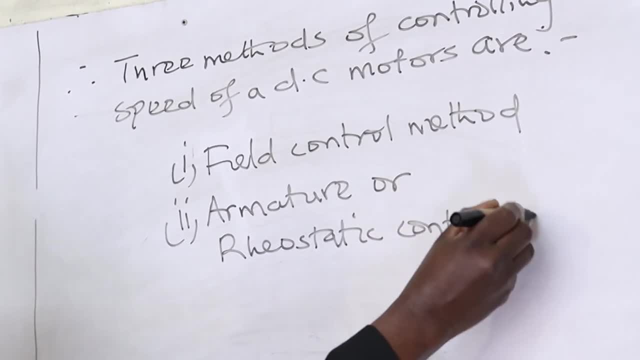 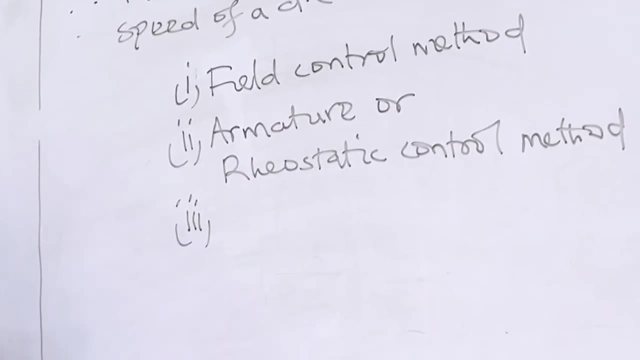 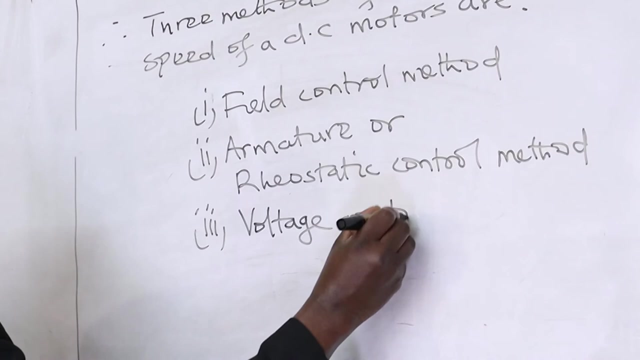 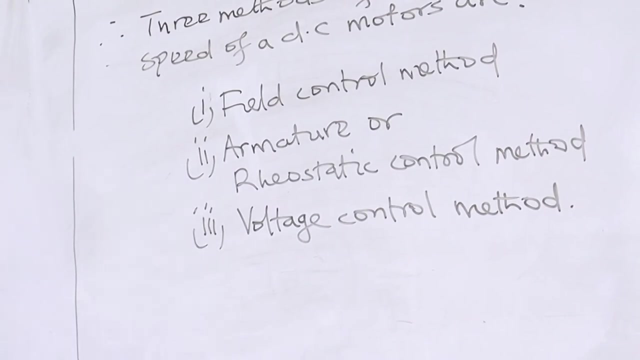 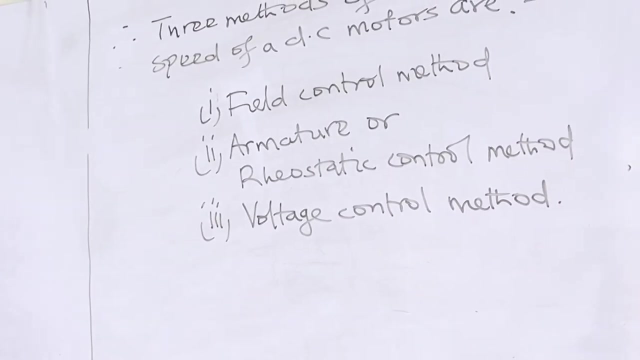 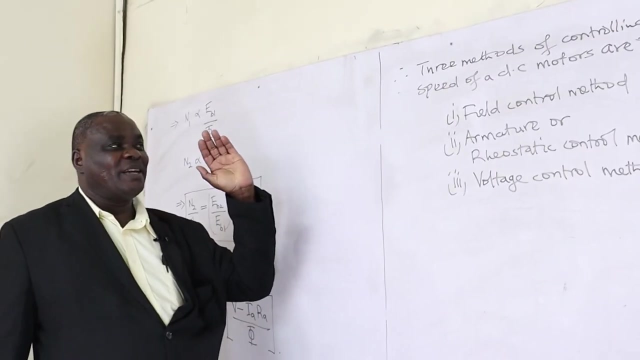 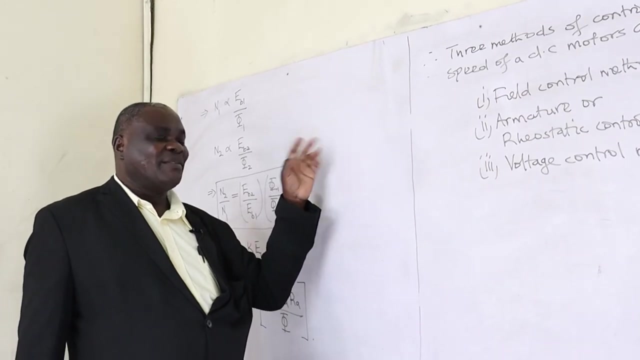 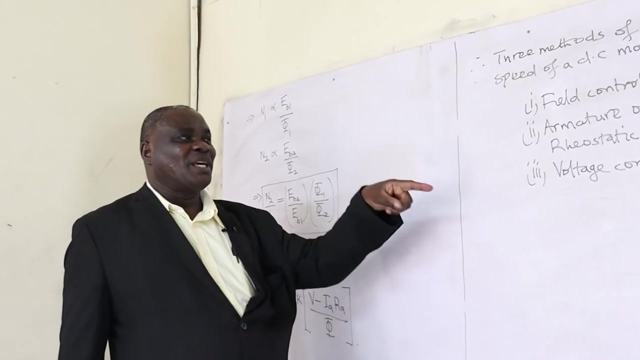 Control method, Training Voltage control method. So from these three methods we would like to see how can we control the speed of various DC motors. We have DC motors, we have the series motor and the shunt motors. How can we control the speed of a shunt motor or a series motor with field control method? 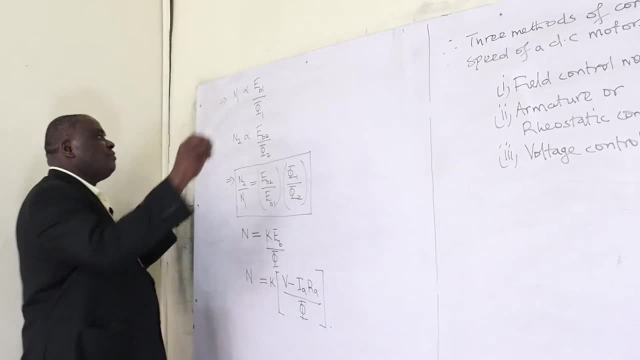 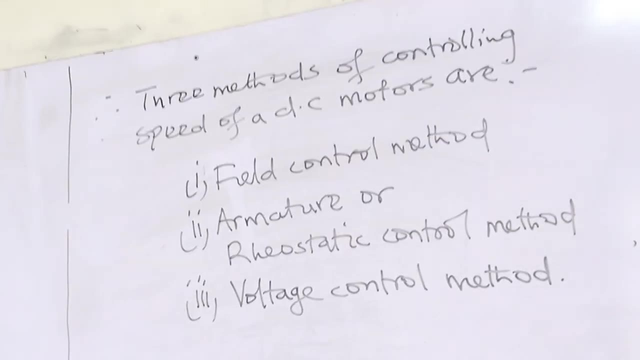 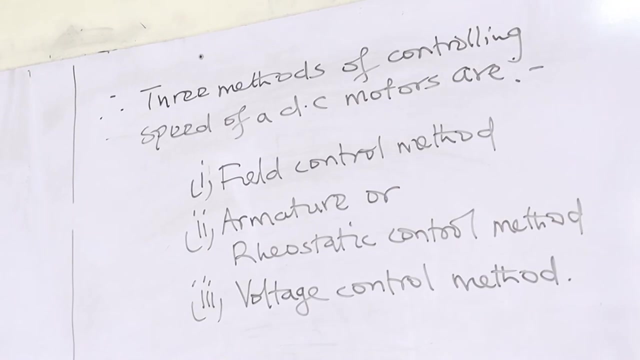 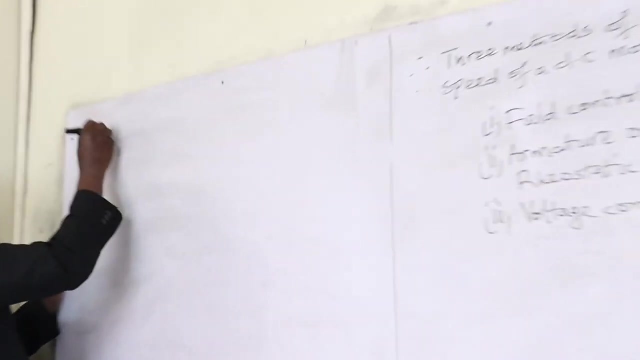 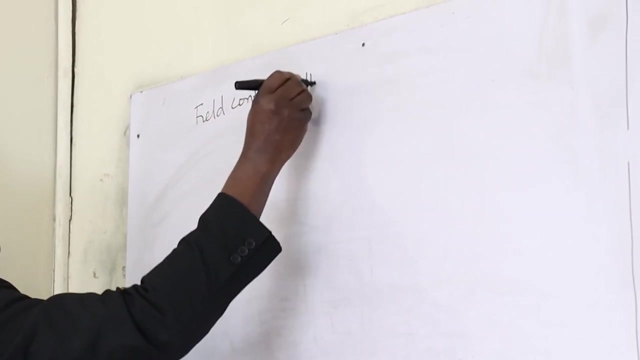 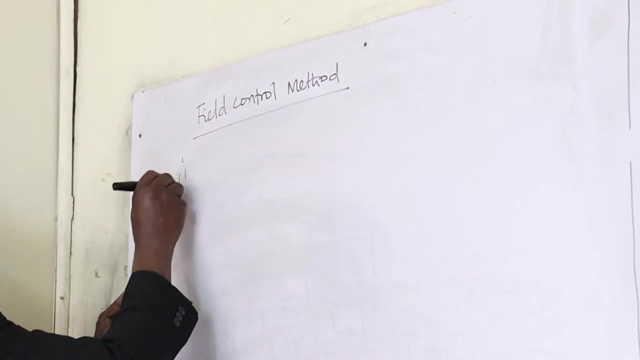 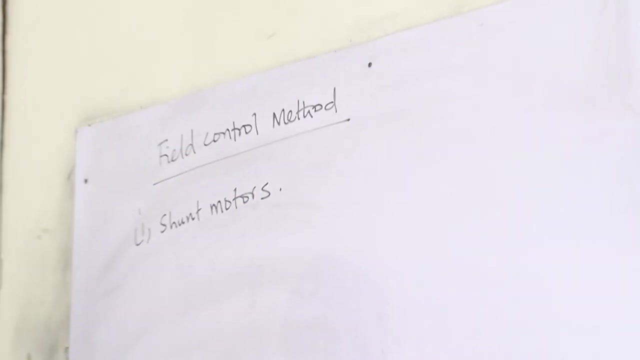 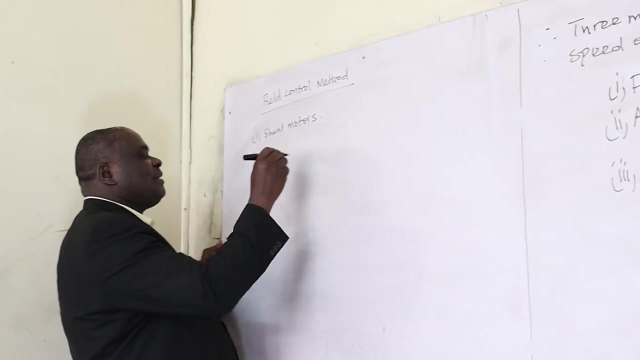 So we now move to In the field control method for shunt motors, a rail shunt is normally inserted in the field circuit of the shunt motor, Of a DC shunt motor, As can be shown in the diagram below. As can be shown in the diagram below. 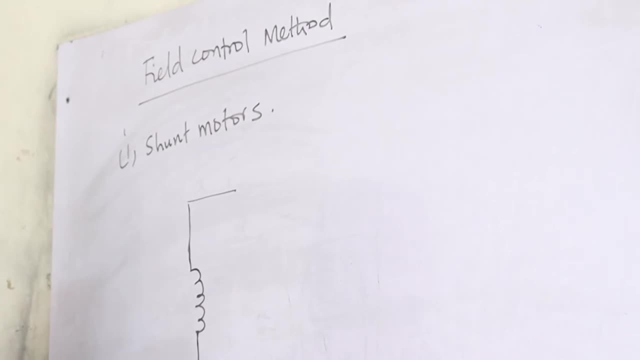 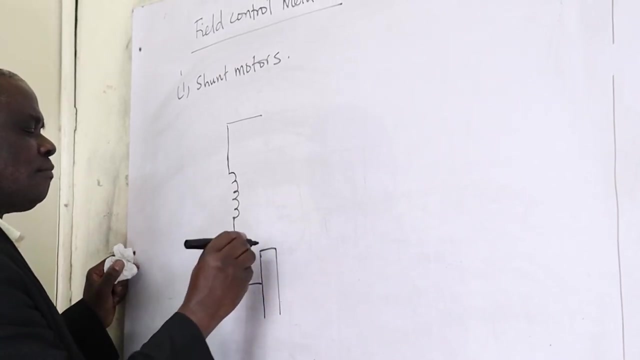 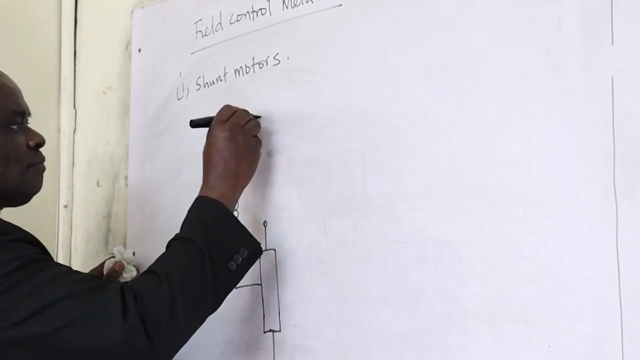 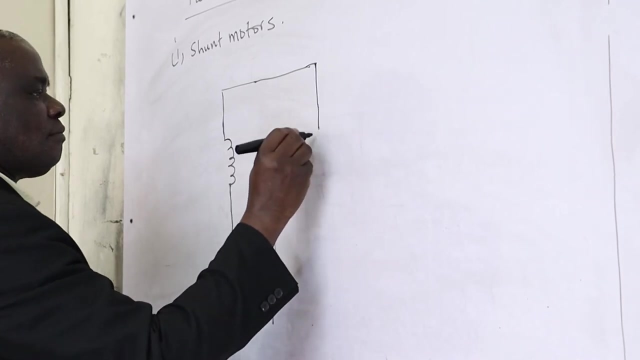 OK, Now we can see, in the domain of a normal shunt motor running on a rotation, a shift of the new movement of the shunt motor From the shunt motor, a shift of the new movement, The shift of the new movement. 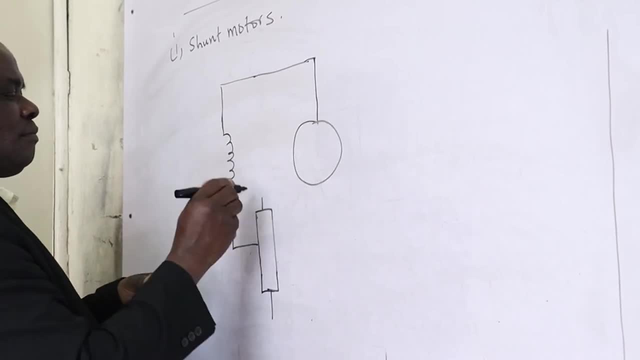 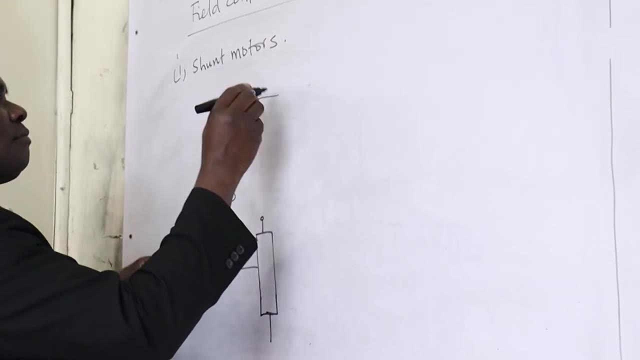 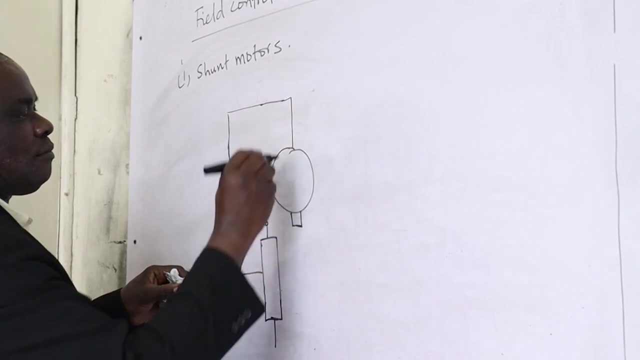 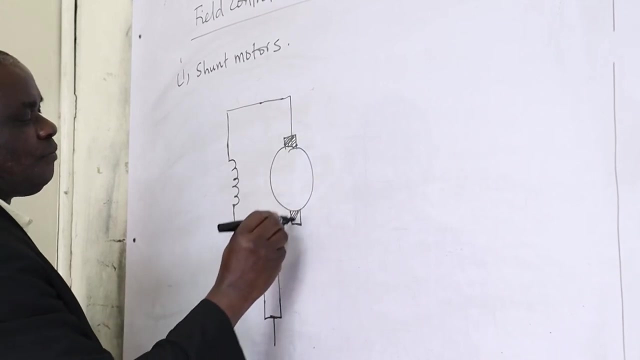 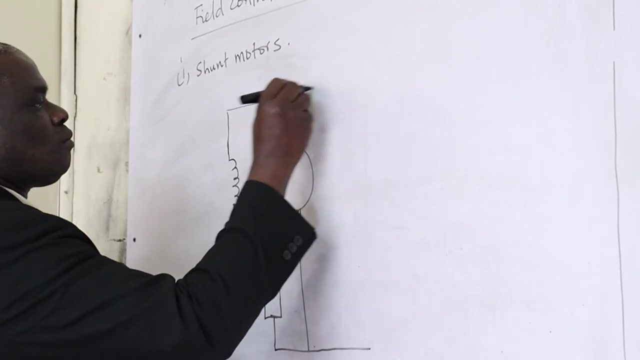 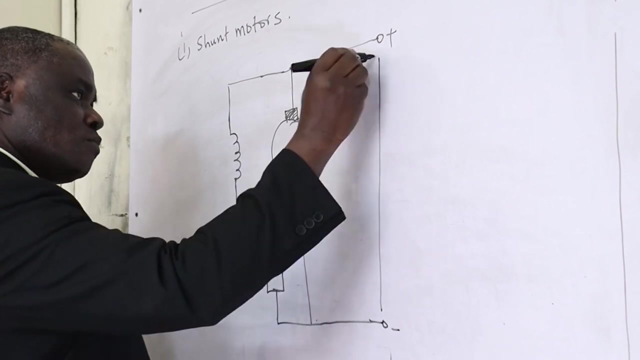 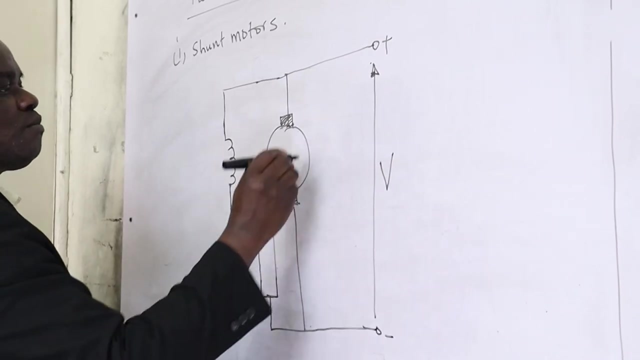 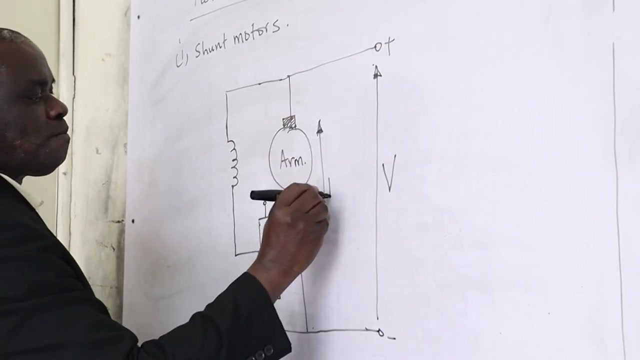 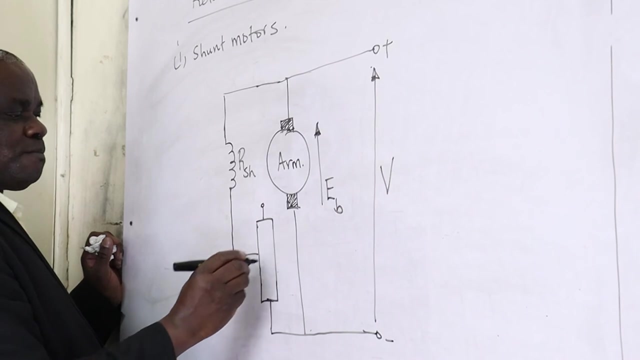 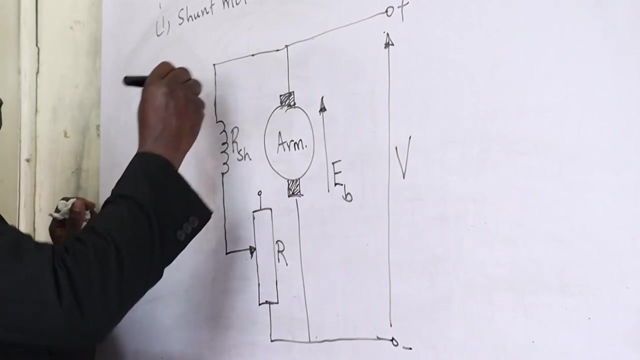 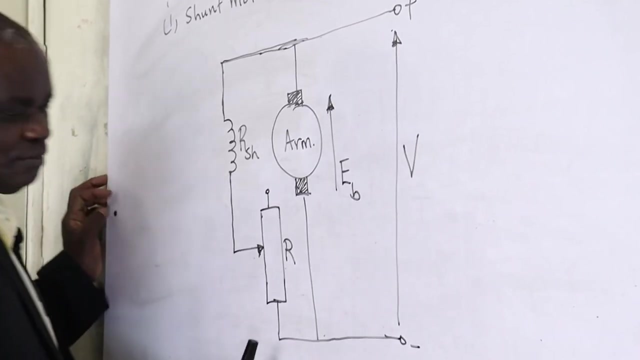 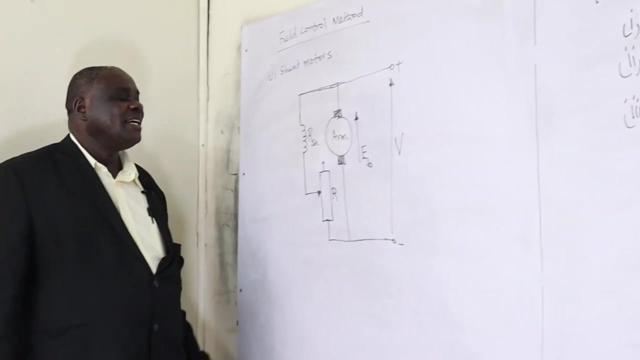 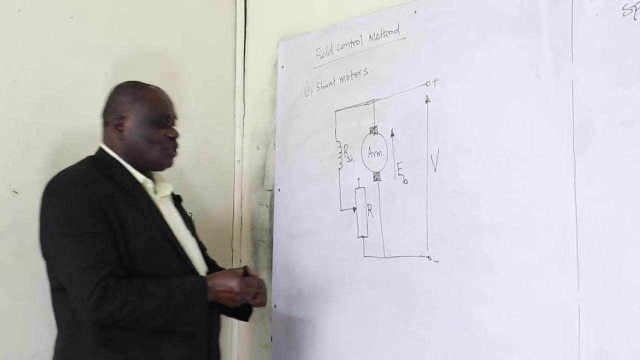 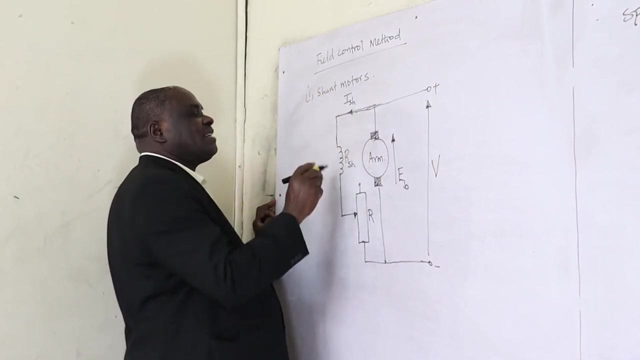 Is there any изменement? Thank you, Thank you. So R that we have here is the rheostat that is inserted in this particular field circuit so as to control the current flow rate. So R is flowing through the field circuit which we will call isent. 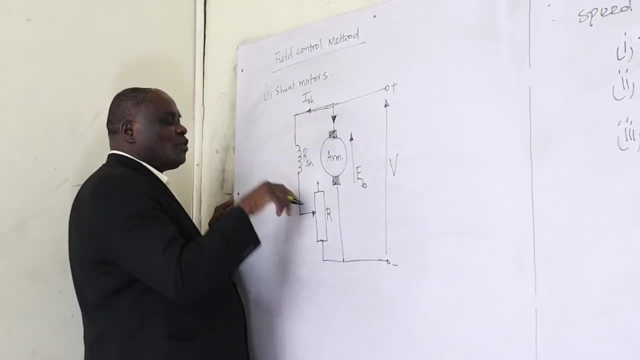 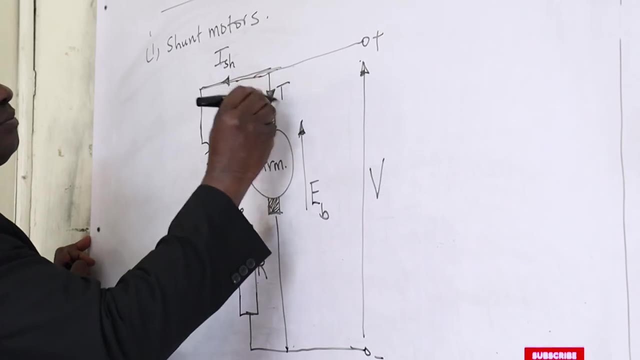 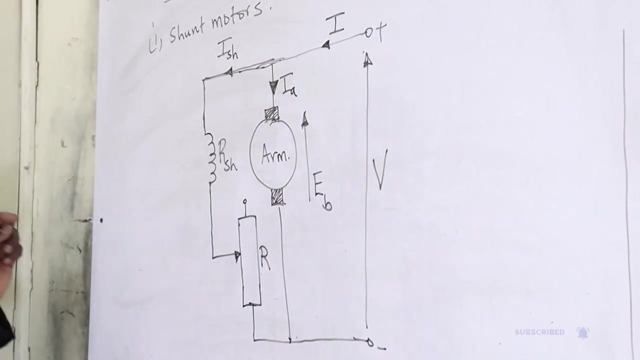 Now, when we control isent, we'll be controlling the flux produced by the field coil, By the field coil. So from this it can be seen this will now be called isent 2.. This will be I2.. 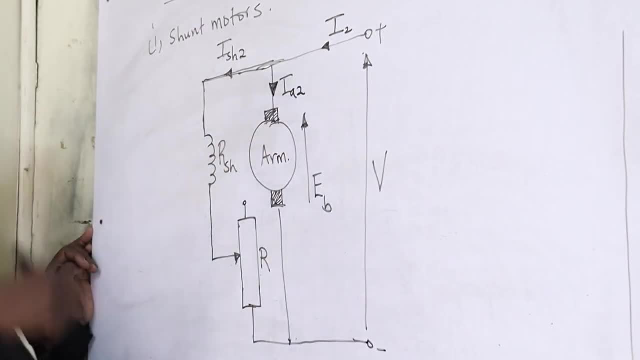 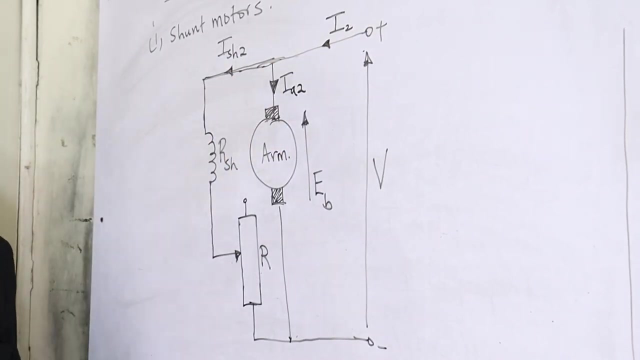 And this will be IA2.. Because originally there was no this rheostat in this particular circuit. By that time we had isent 1 flowing, We had I1 drawn from the supply, We had IA1 flowing and through there the MRC. 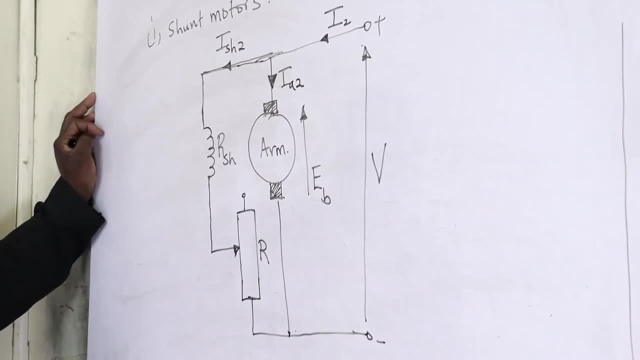 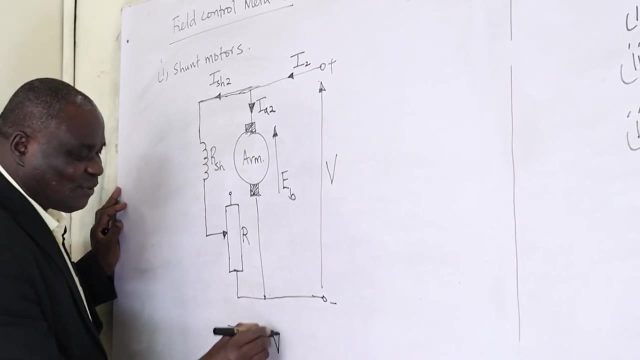 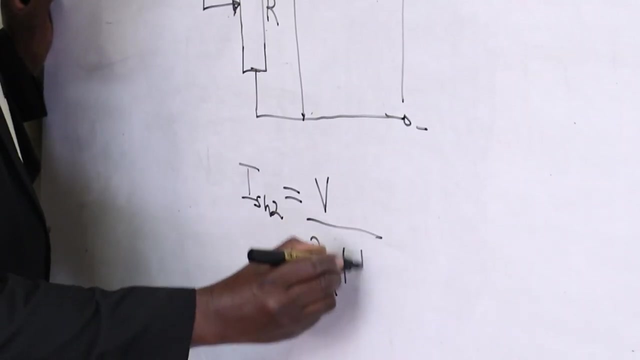 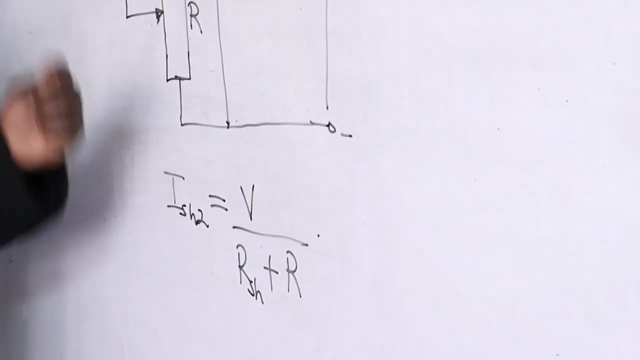 Now, from this indication it can be seen now for us to obtain isent 2.. Isent 2 will be equal to V divided by R'sent plus R, R'sent plus R. This isent 2 will be responsible. 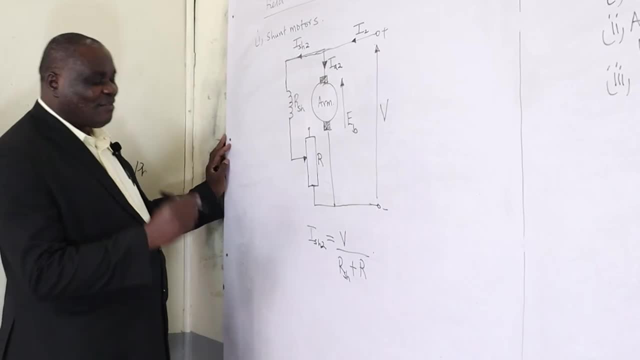 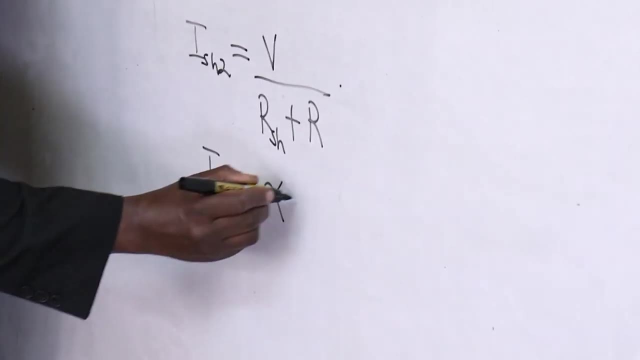 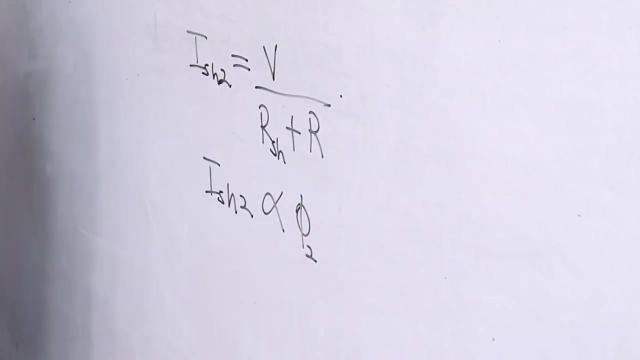 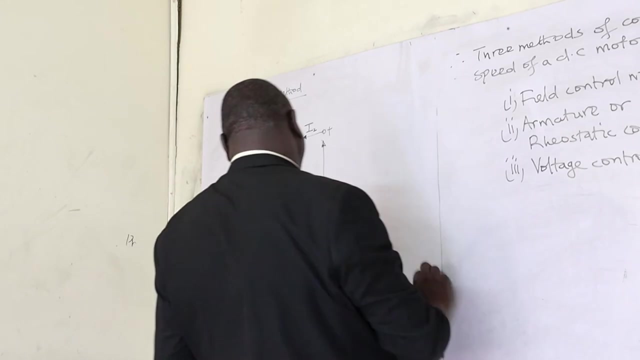 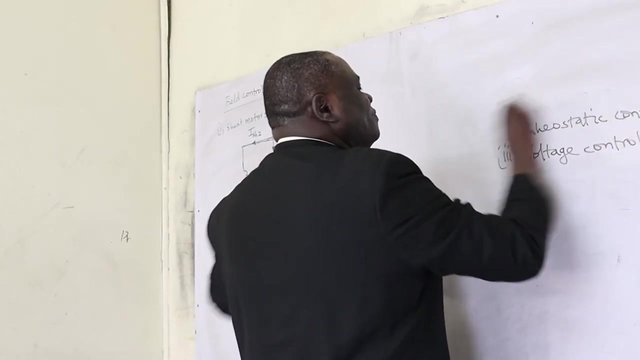 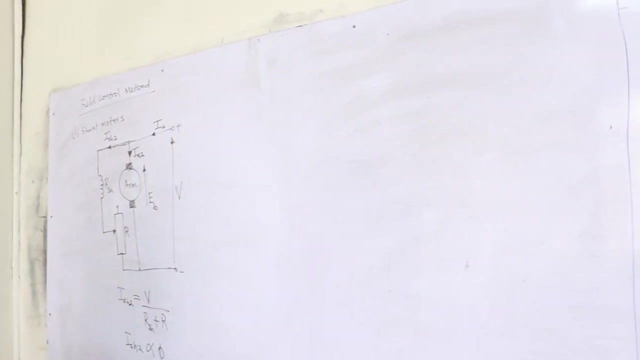 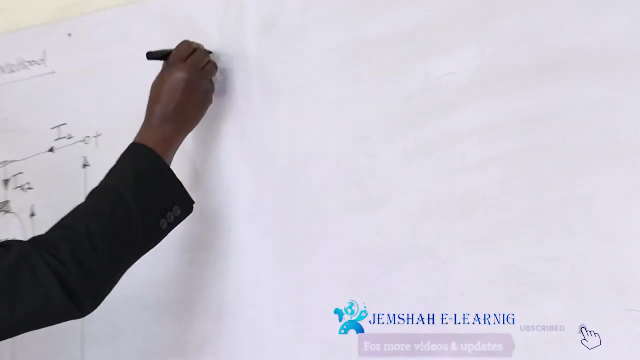 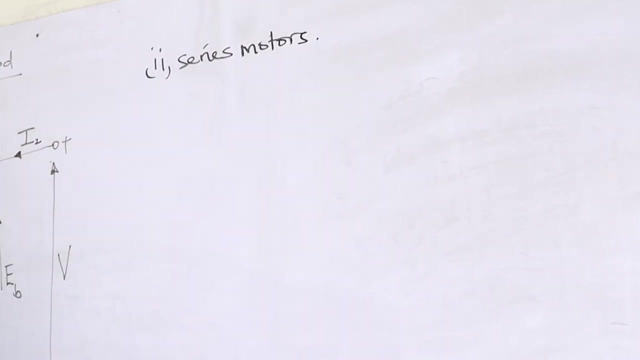 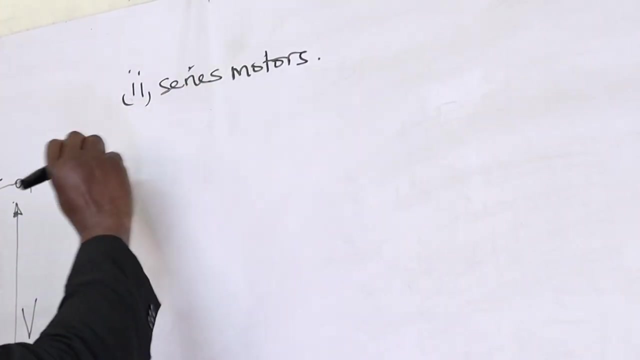 product, for production, for production fraction of our phi two. So I shunt two will be proportional to phi two before the circuit, before the magnetic circuit is saturated. For series mortars we have got some methods of controlling the flux in the DC series circuit. 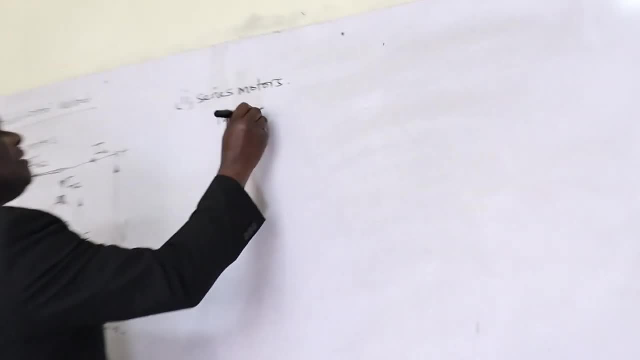 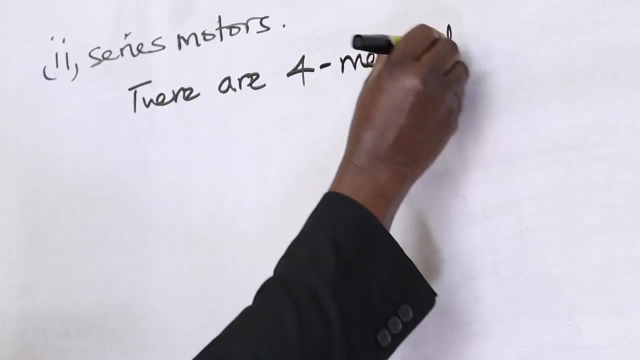 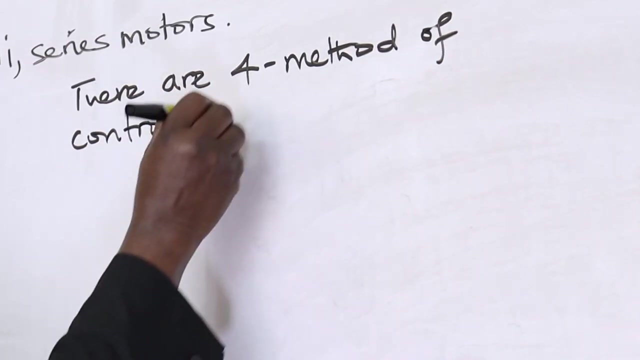 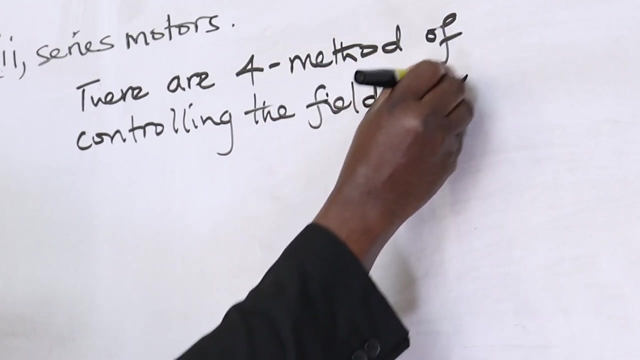 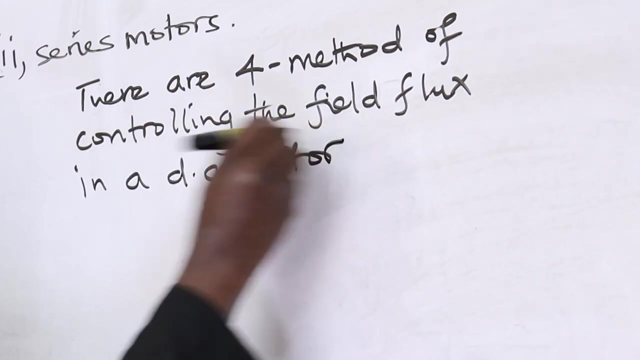 So there are four methods, Okay, Okay, So there are four methods of controlling the field flux in a DC series: motor One, Two, Three, Four, Five, Six, Seven, Eight, Nine, 10., 11., 12.. 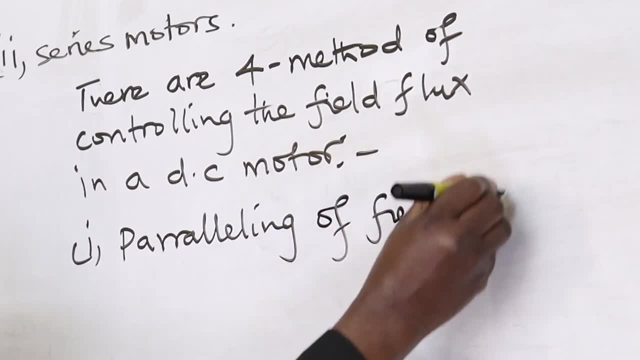 13., 14., 15., 16., 17., 18., 19., 20., 21., 22., 23., 24., 25., 26., 27., 28., 29.. 30., 31., 32., 33., 33., 34., 35., 36., 37., 38., 39., 40., 41., 42., 43., 44., 44.. 45., 46., 46., 47., 48., 49., 50., 51., 52., 53., 52., 53., 54., 55., 56., 57., 58.. 59., 60., 61., 62., 63., 63., 64., 65., 66., 67., 68., 67., 68., 69., 69., 70., 71.. 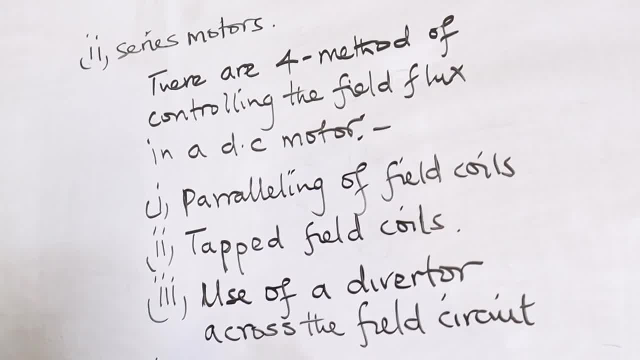 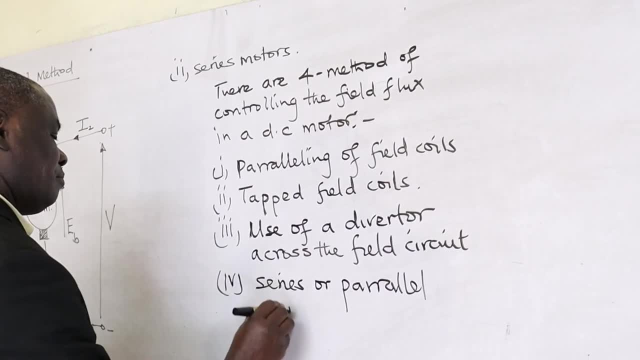 72., 72., 73., 74., 75., 76., 76., 77., 78., 79., 80., 81., 82., 83., 84., 85., 86..